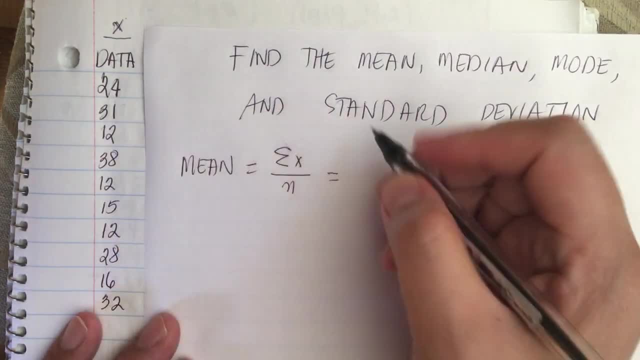 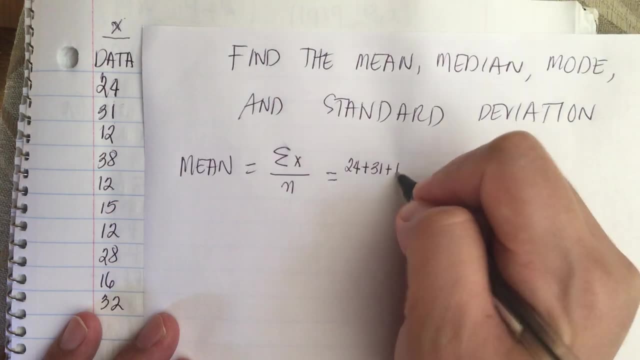 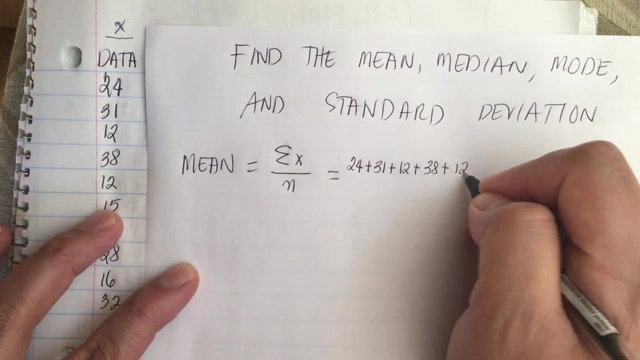 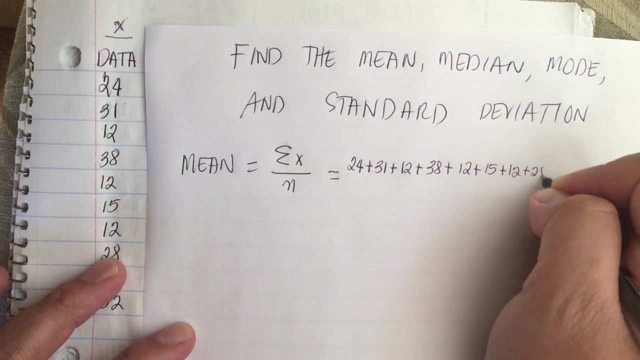 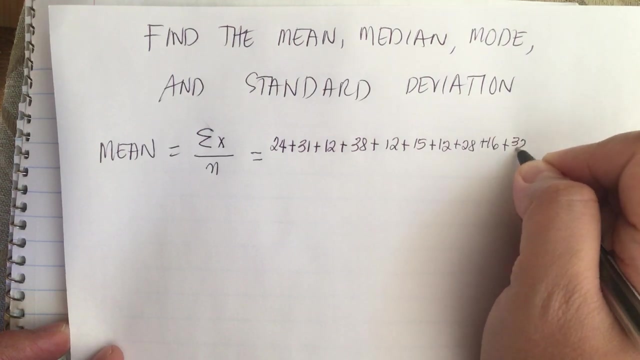 So this is equal to: so we have 24.. Plus 31, plus 12,, plus 38,, plus 12,, plus 15,, plus 12,, plus 28,, plus 16, plus 32.. So now this is divided by: 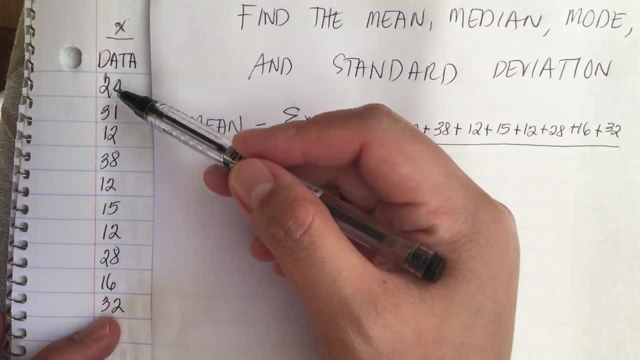 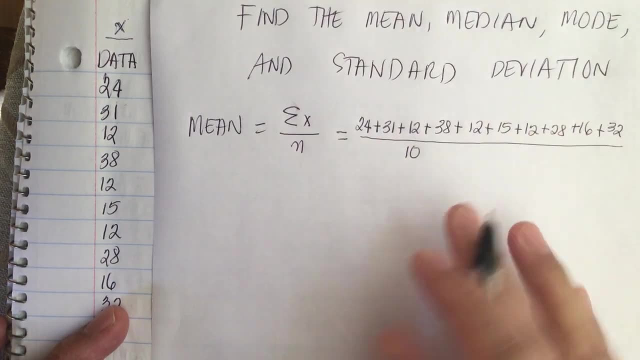 N, or the total number of data. So we have 1,, 2,, 3,, 4,, 5,, 6,, 7,, 8,, 9,, 10.. So we have 10 data points. 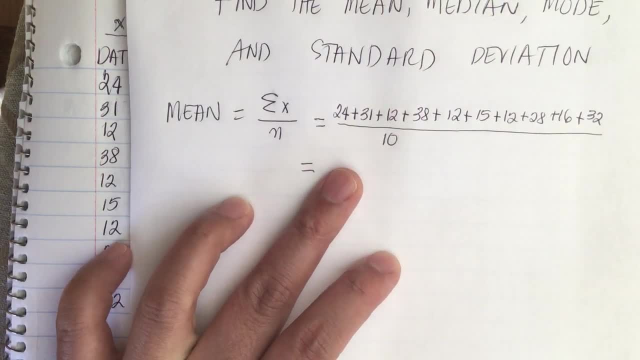 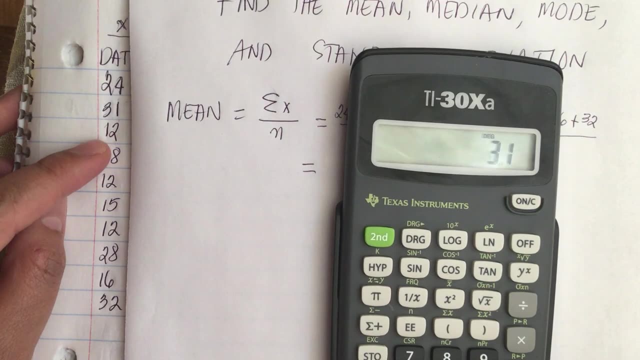 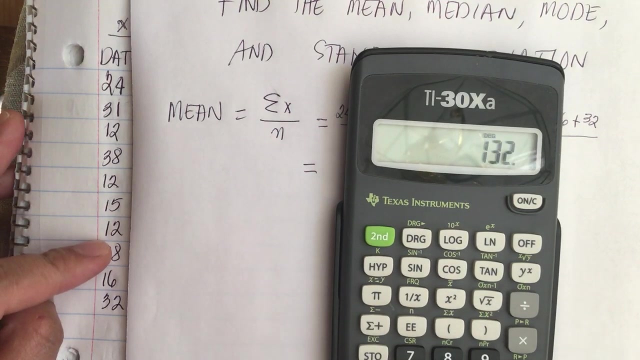 So this is equal to, so we use our calculator. So we have 24, plus 31, plus 12, plus 38, plus 12, plus 15.. Plus 12, plus 28,, plus 16, plus 32.. 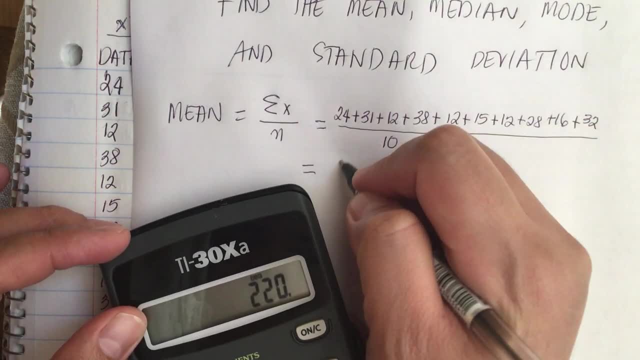 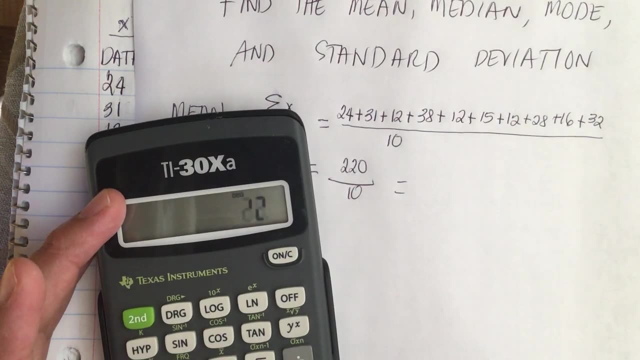 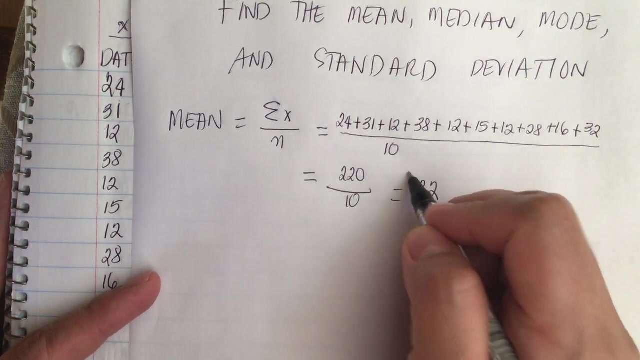 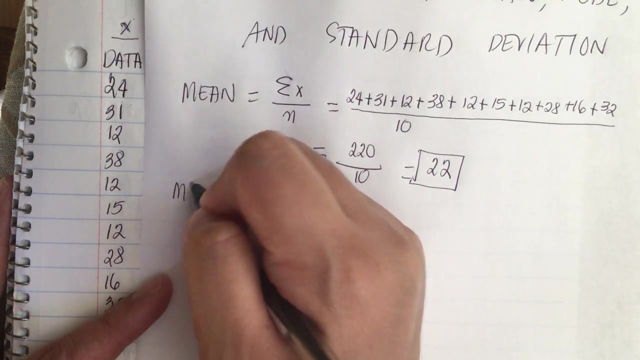 And this is equal to 220.. And this is divided by 10.. So this is equal to 22.. So the mean is equal to 22.. So this is the mean. So now to find the median. Oh, it's going down and backwards. 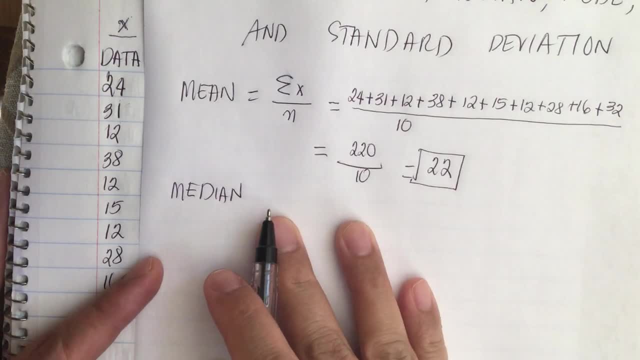 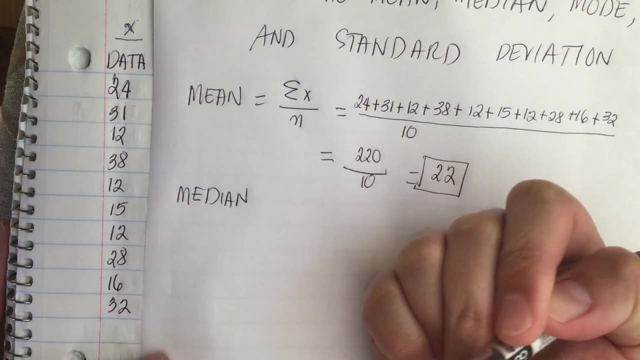 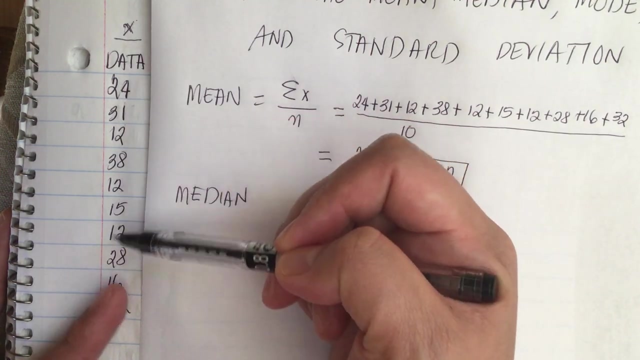 So median. So to find the median, the median is the number in the middle. So we have this and the number in the middle is the median. But first, since the row data X is not arranged in ascending order, so we have to do that first. 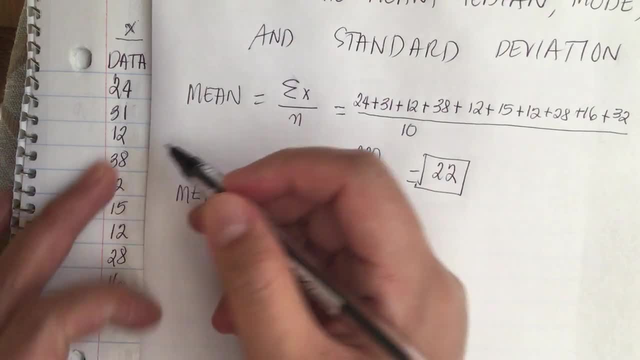 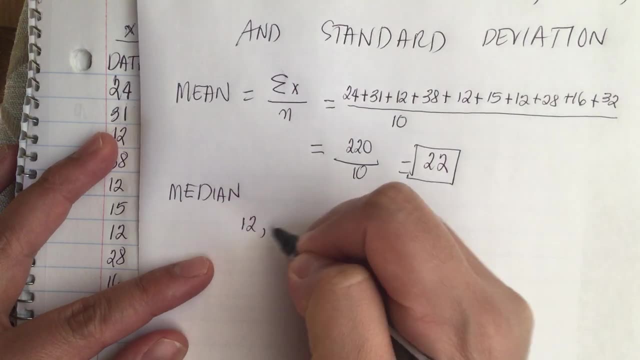 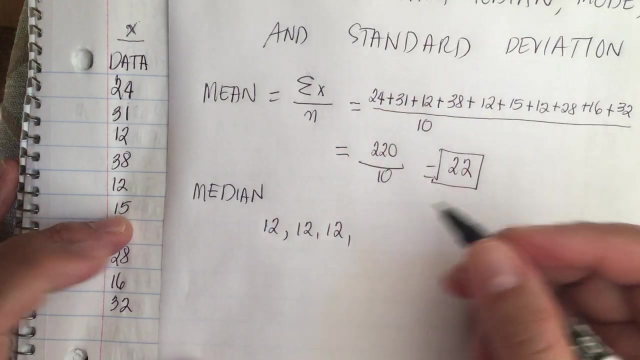 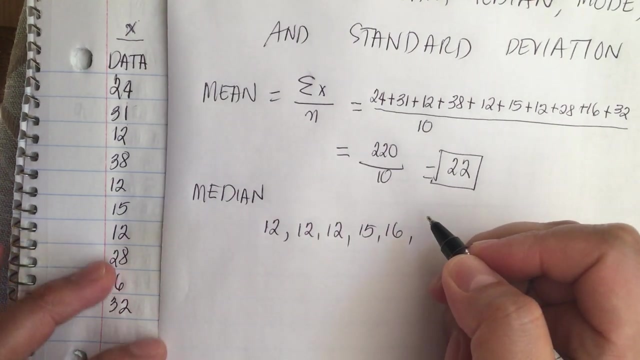 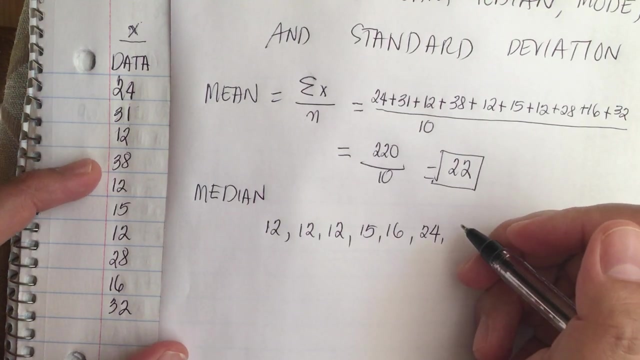 So we have? we have how many? 12,, 1,, 2,, 3.. So we have 12,, 12,, 12, and then we have 15,, we have 16, and then we have 24, and then 28.. 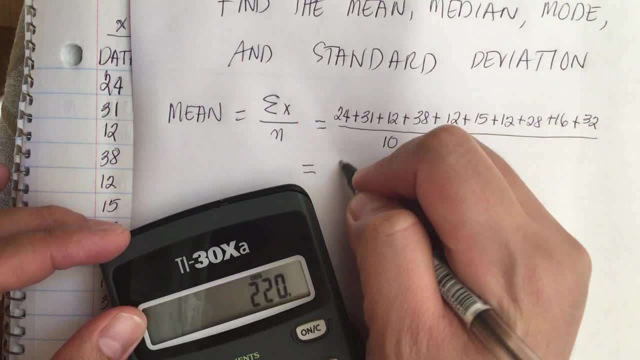 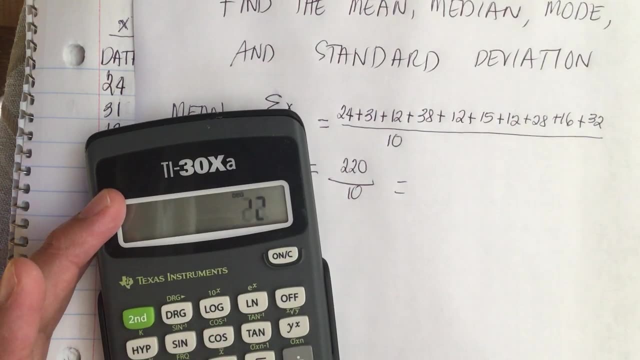 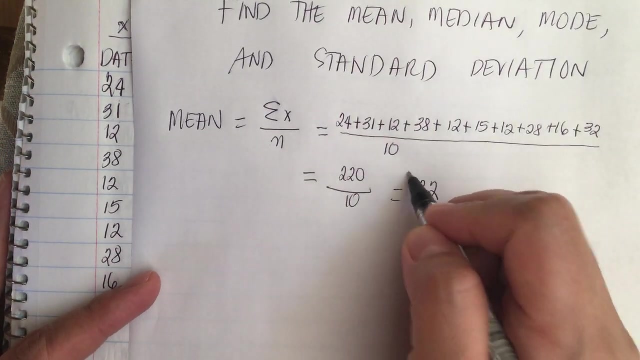 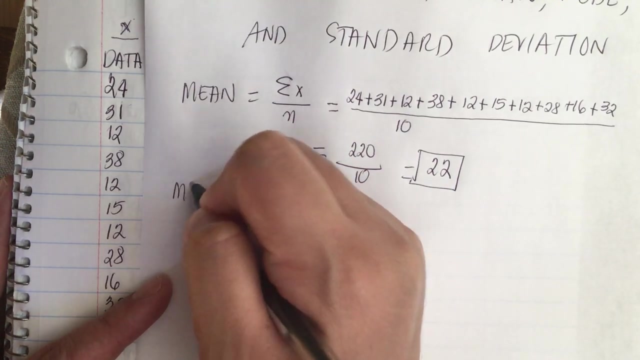 And this is equal to 220.. And this is divided by 10.. So this is equal to 22.. So the mean is equal to 22.. So this is the mean. So now to find the median. Oh, it's going down and backwards. 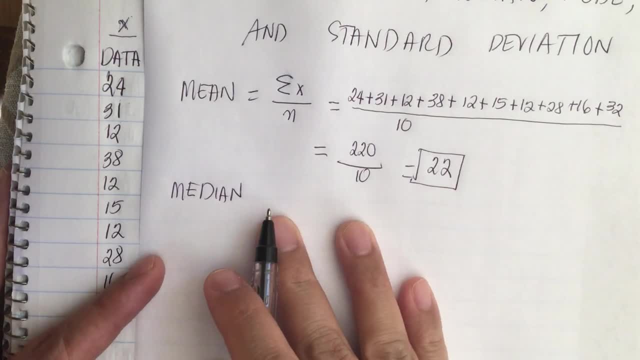 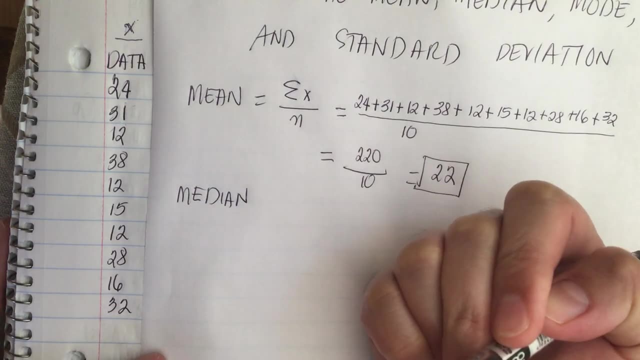 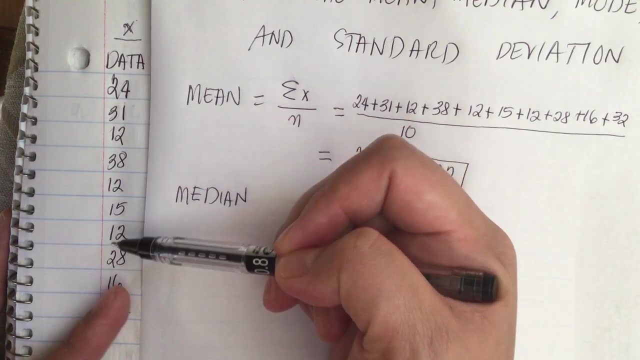 So median. So to find the median, the median is the number in the middle. So we have this and the number in the middle is the median. But first, since the row data X is not arranged in ascending order, so we have to do that first. 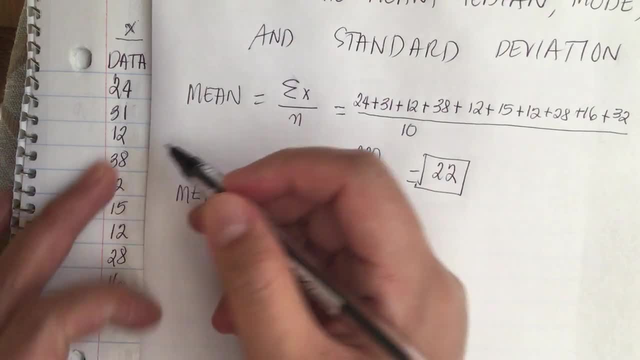 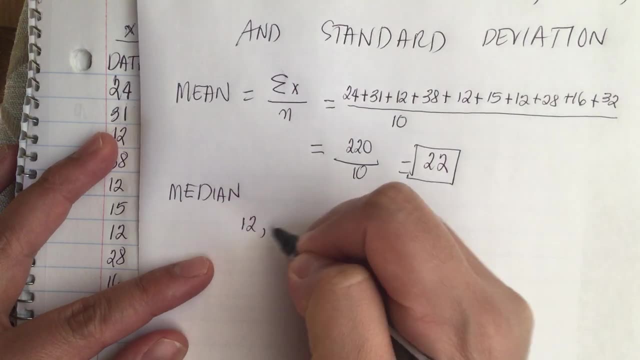 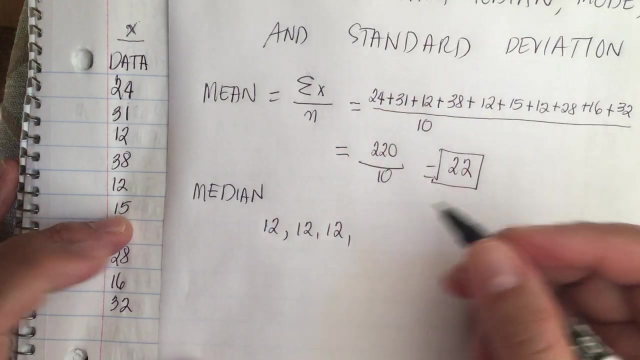 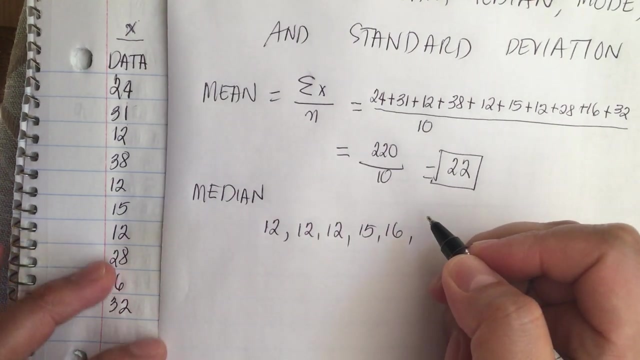 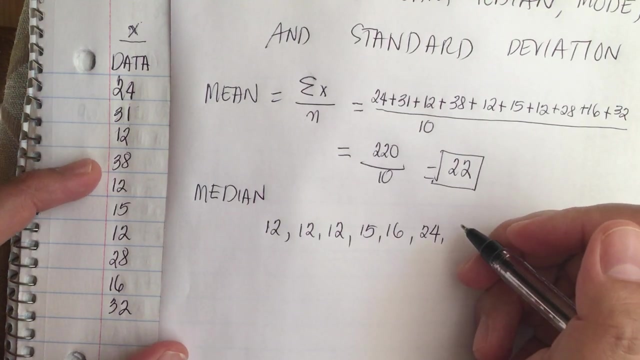 So we have? we have how many? 12,, 1,, 2,, 3.. So we have 12,, 12,, 12, and then we have 15,, we have 16, and then we have 24, and then 28.. 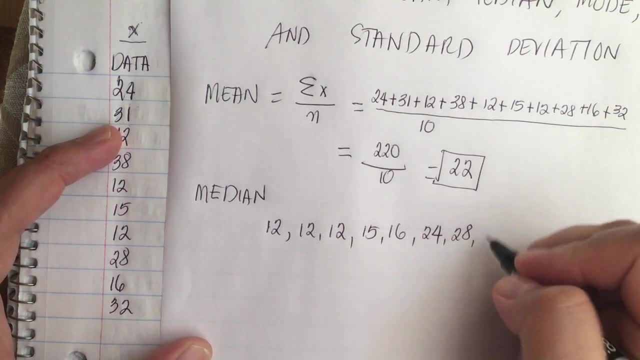 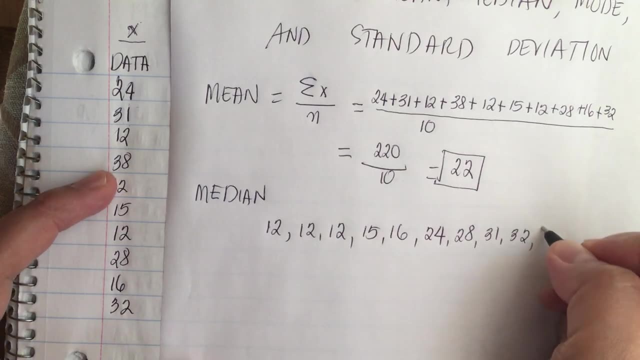 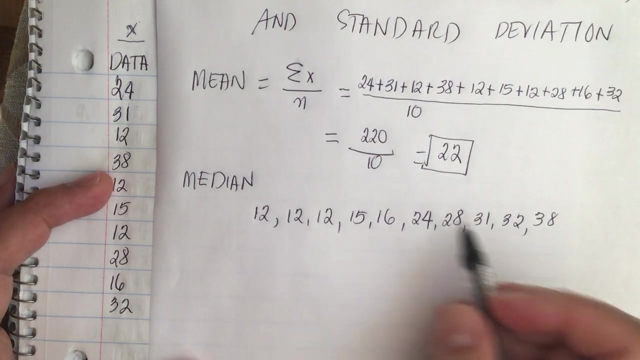 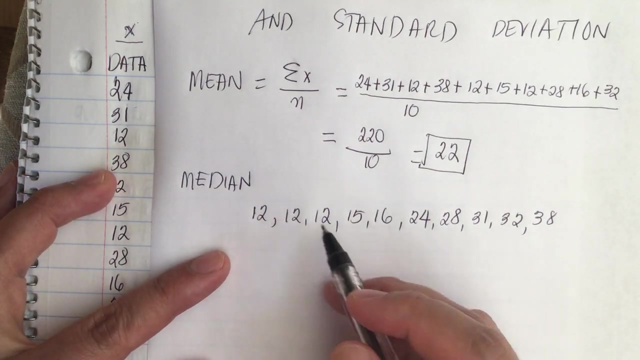 And then 31,, 32,, and then 38,, 2,, 4,, 6,, 8,, 10.. So we list the data in ascending order. So now the number in the middle is the median. So since this is an even number, so the number the two, we take the two numbers in the 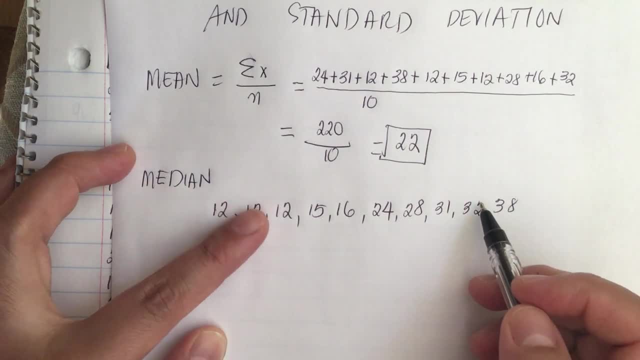 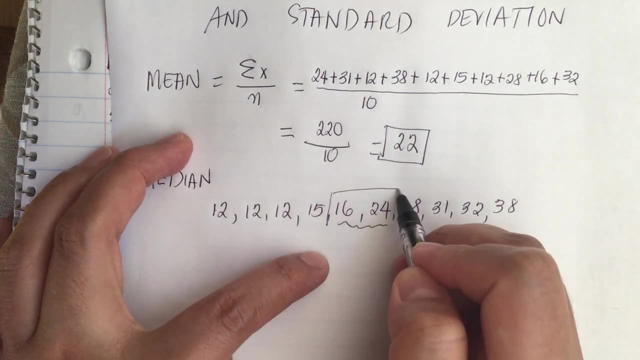 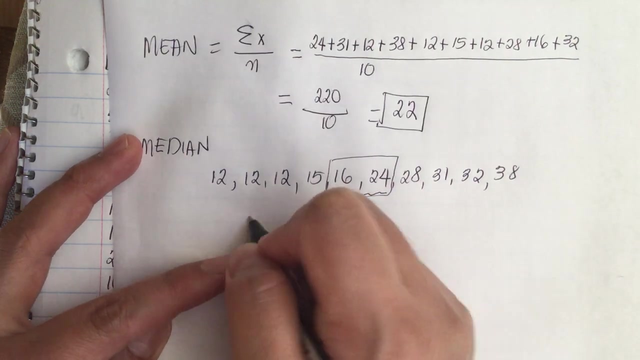 in the middle. So we have. so the number in the middle is 16 and 24.. So, since this is an even number of data points, so we have 16 plus 24, and we divide it by 2,. 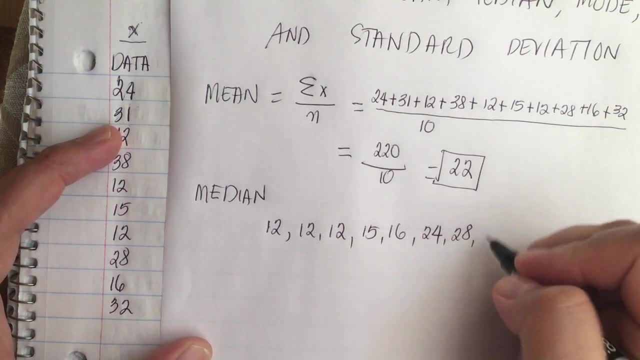 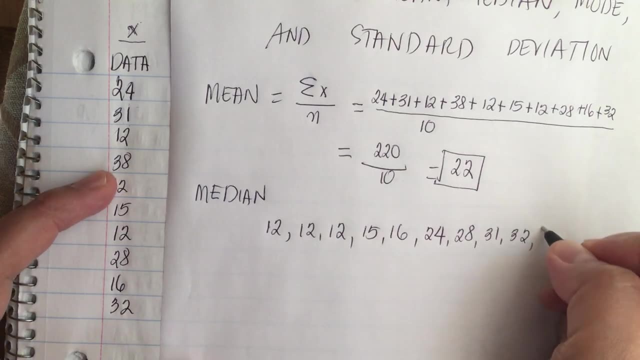 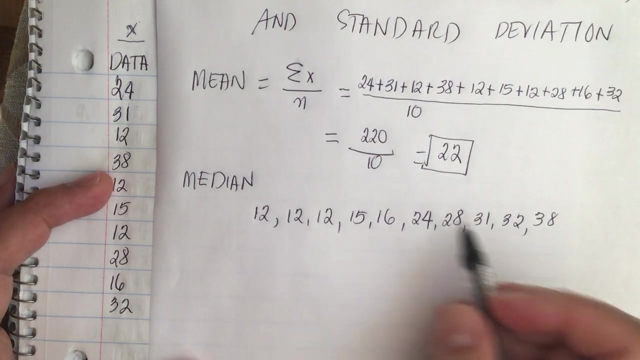 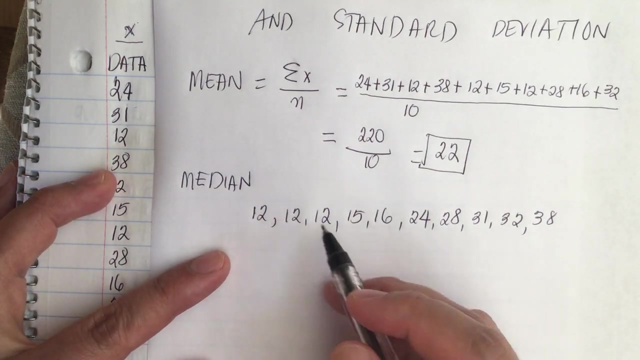 And then 31,, 32,, and then 38,, 2,, 4,, 6,, 8,, 10.. So we list the data in ascending order. So now the number in the middle is the median. So since this is an even number, so the number the two, we take the two numbers in the 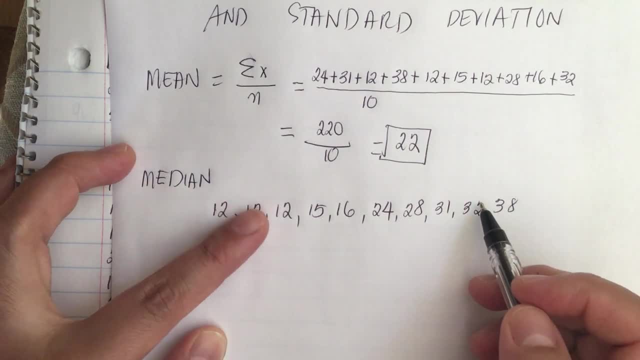 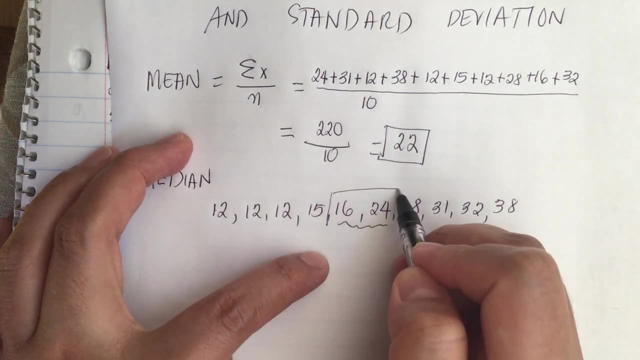 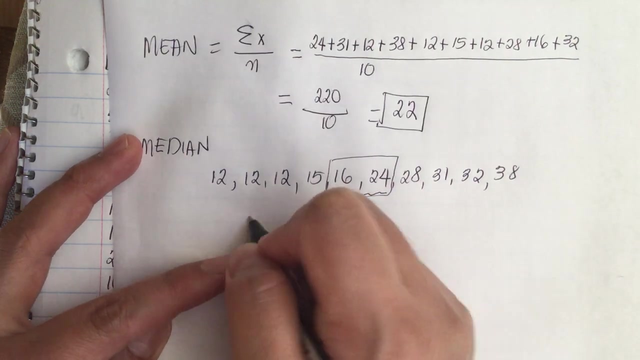 in the middle. So we have. so the number in the middle is 16 and 24.. So, since this is an even number of data points, so we have 16 plus 24, and we divide it by 2,. 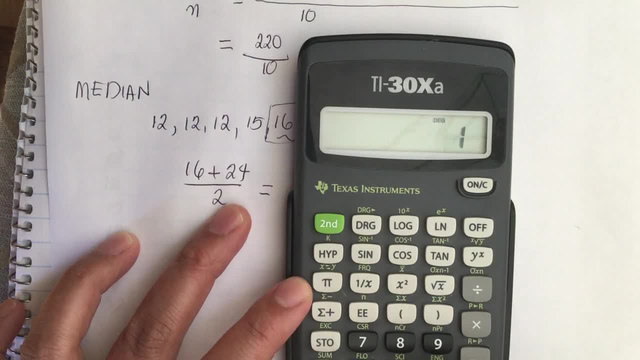 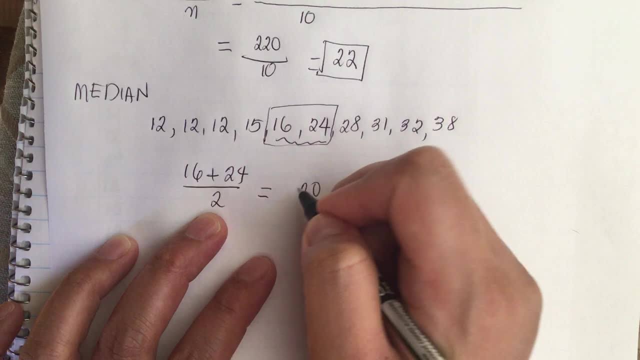 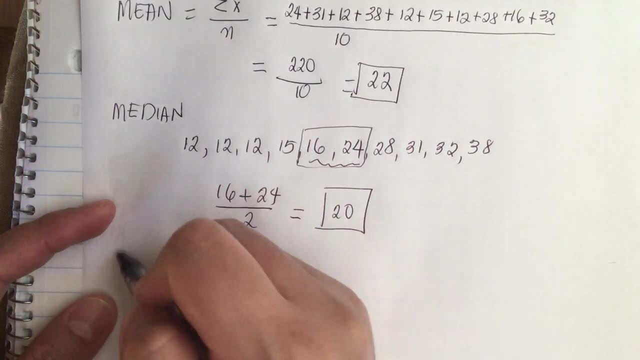 and this will give us the median. So we have 16 plus 24, divide 2.. So this is 20.. So the median is 20.. So and the mode: the mode is the most popular number. 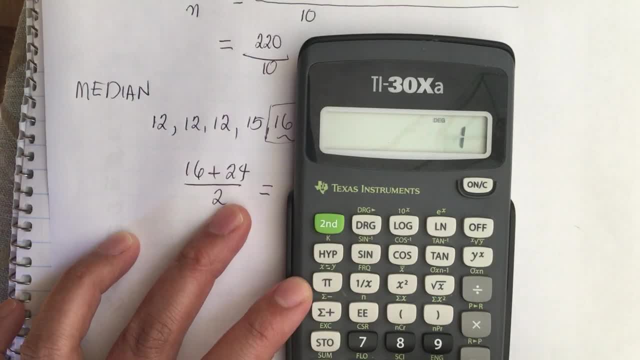 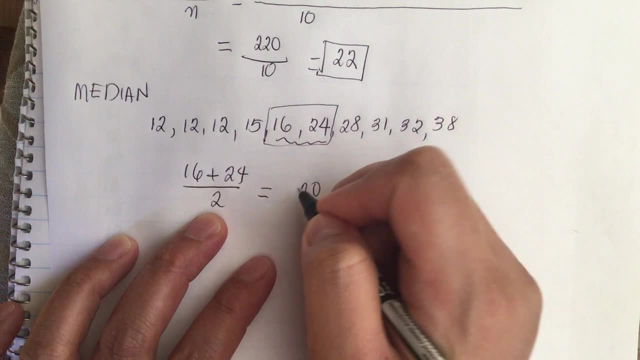 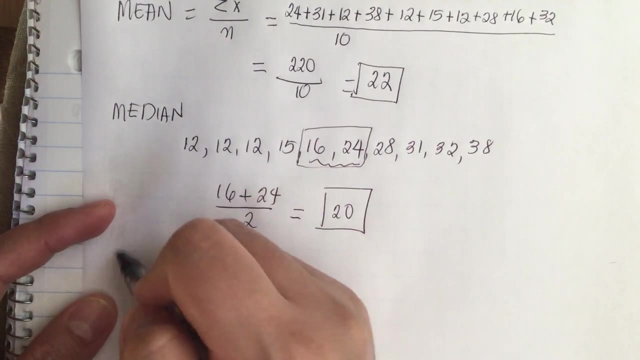 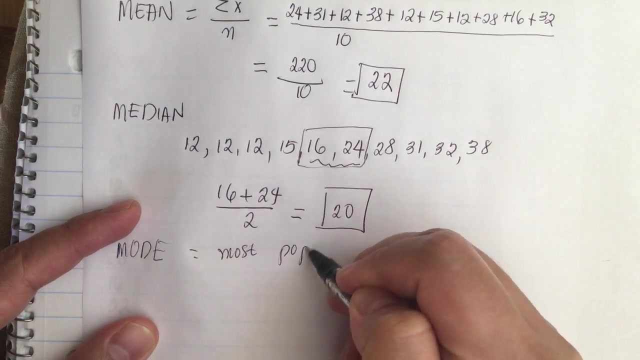 and this will give us the median. So we have 16 plus 24, divide 2. It's 20.. So the median is 20.. So and the mode? the mode is the most popular number, The most popular number. 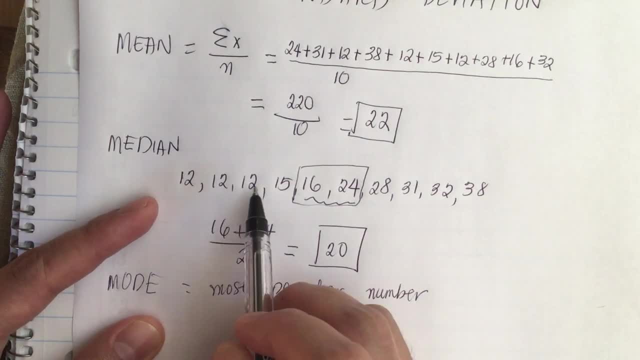 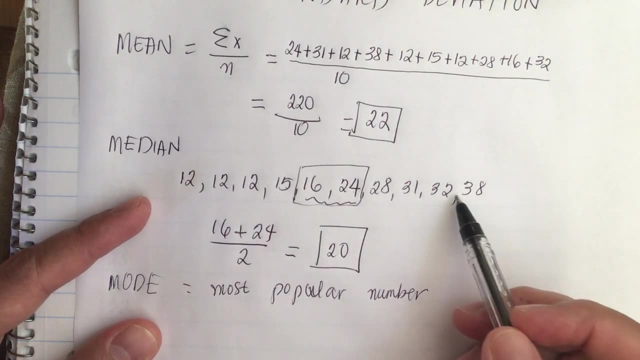 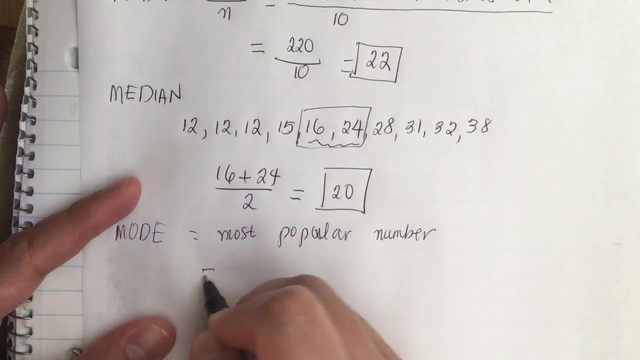 So the most popular number is 12, because there are three of them. So there are three 12s, one, 15.. 16, 124, 128, 132, 131 and 138. so the most most popular number is 12, so mode is equal to 12.. 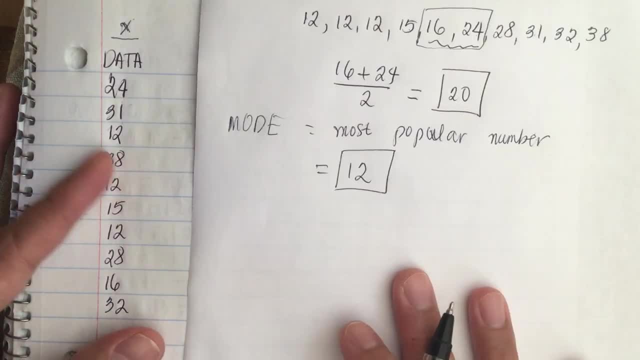 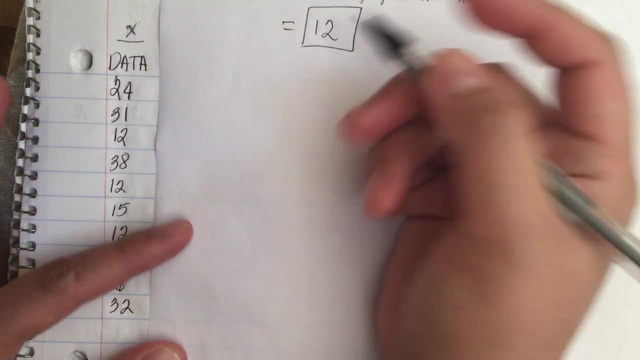 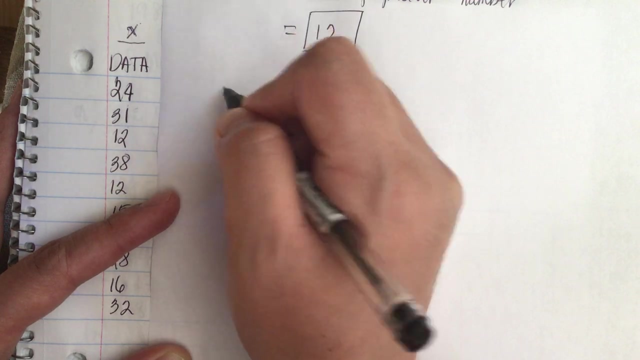 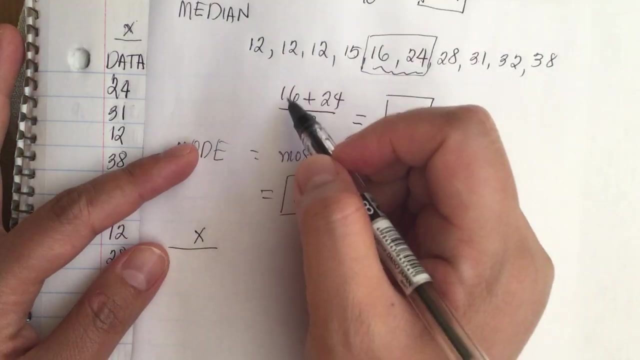 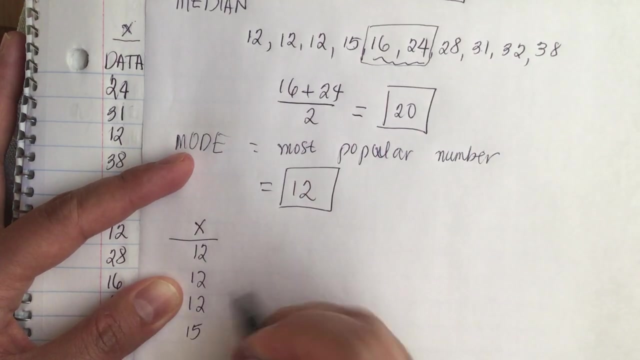 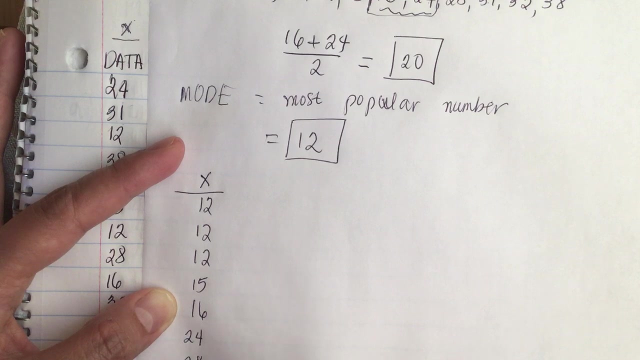 so now to find the standard um deviation, we need to make columns, so we need, so this is x. it's easy, so i just rewrite the um data here. so we have the x and i'm gonna um. do them in ascending order. so we have 12, 12, 12, 15, 16, 24, 28, 31, 32 and 38. so now we have. 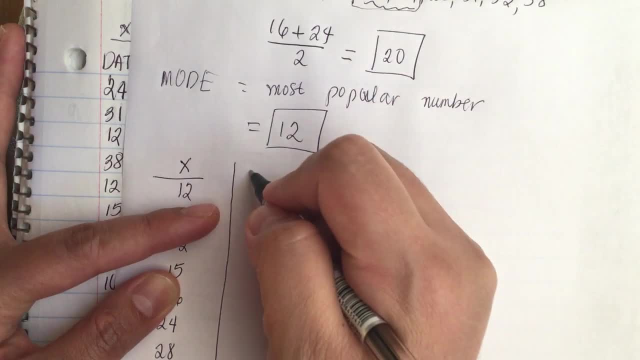 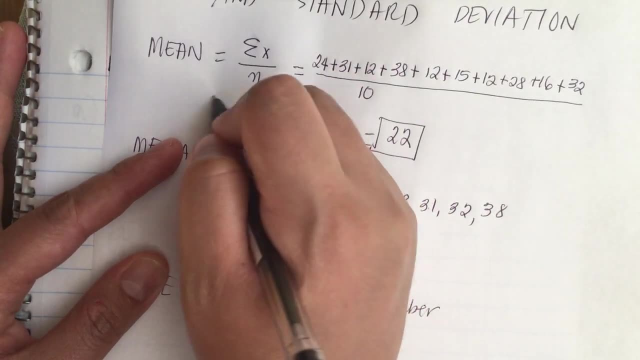 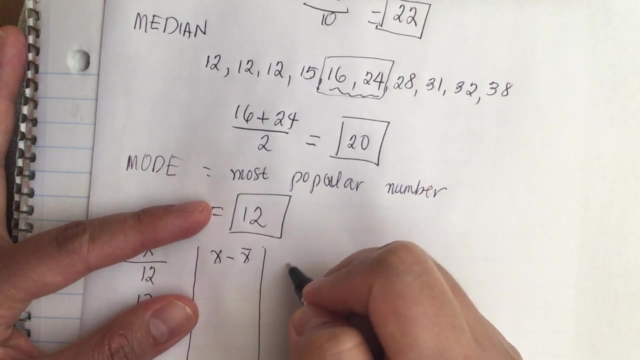 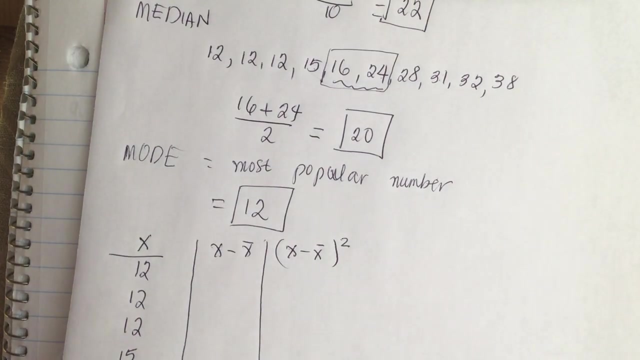 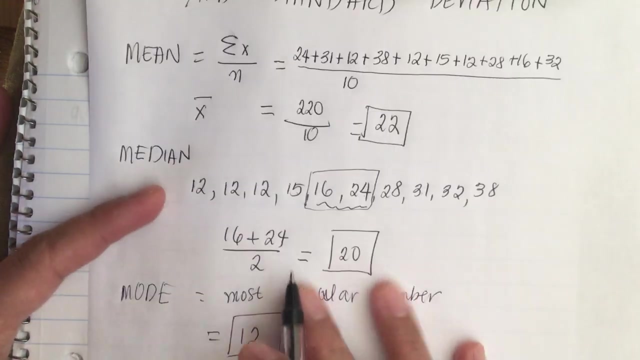 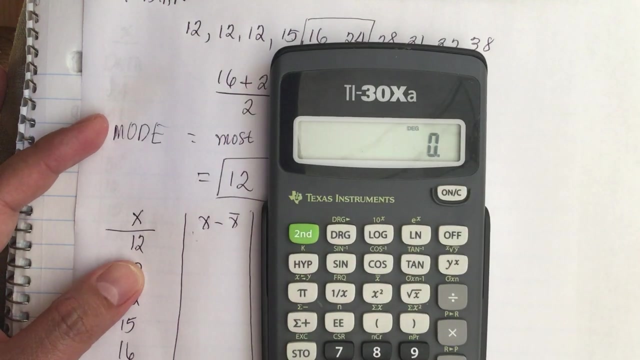 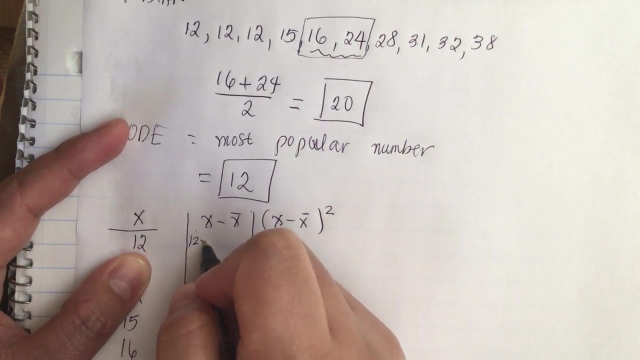 another. we need another column. so we have x minus x bar, or x bar is also called the mean. so this is the mean, x bar means mean. and then we need x minus x bar squared, so now we have 12. so we know that the mean is equal to 22.. so we have 12.. so this is equal to 12.. so x is equal to 12 minus x bar, x bar. 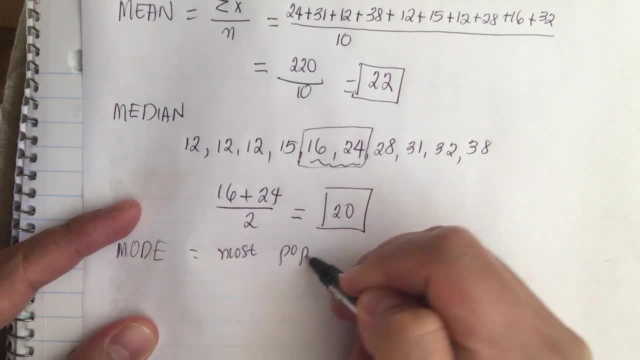 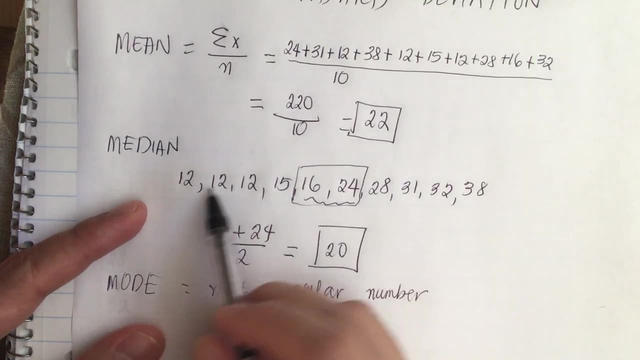 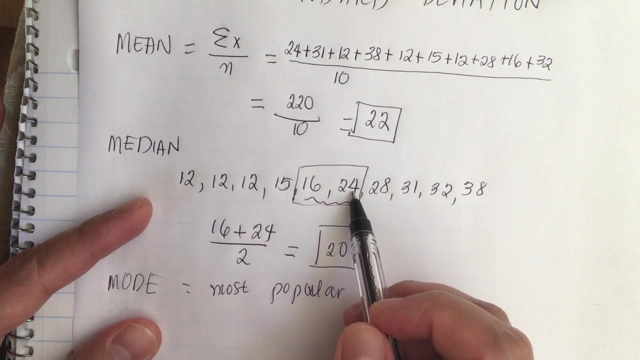 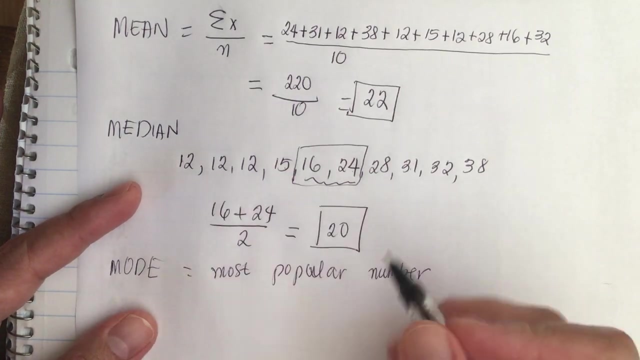 The most popular number. So the most popular number is 12 because there are three of them. So there are three 12s, one 15, one 16.. 16, 124, 128, 132, 131 and 138. so the most most popular number is 12, so mode is equal to 12.. 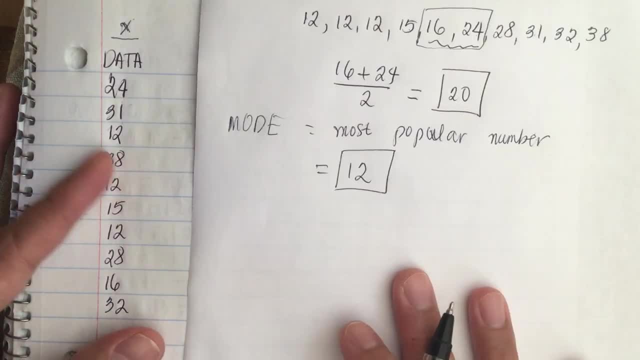 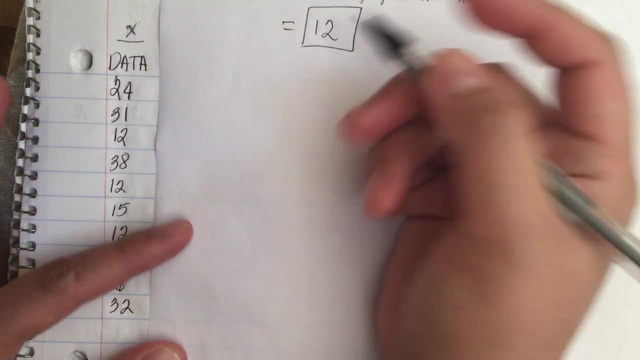 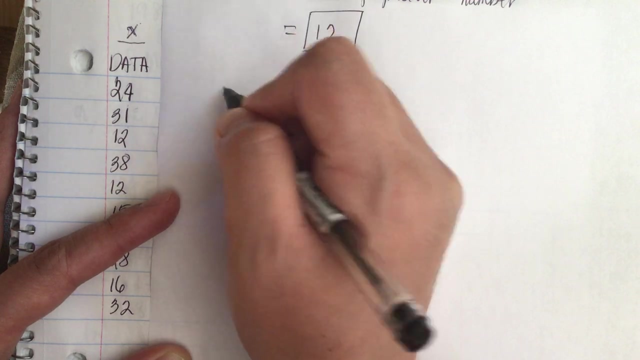 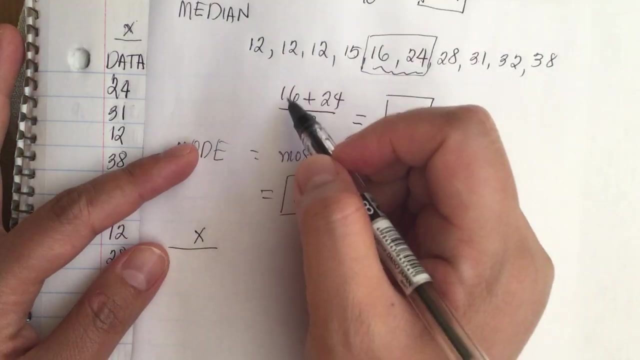 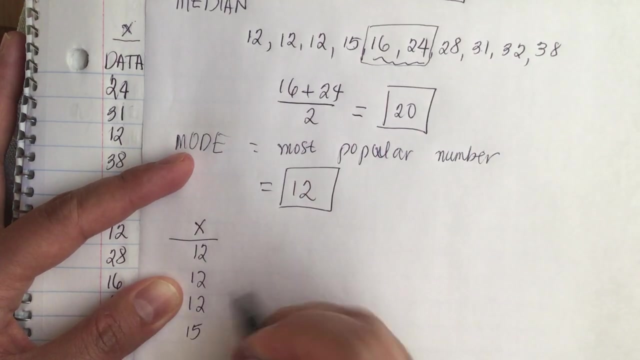 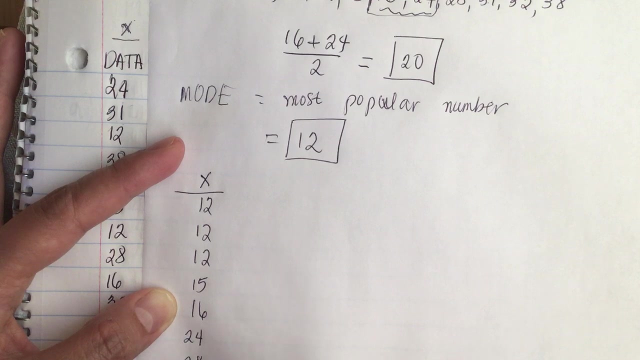 so now to find the standard um deviation, we need to make columns, so we need, so this is x. it's easy, so i just rewrite the um data here. so we have the x and i'm gonna um. do them in ascending order. so we have 12, 12, 12, 15, 16, 24, 28, 31, 32 and 38. so now we have. 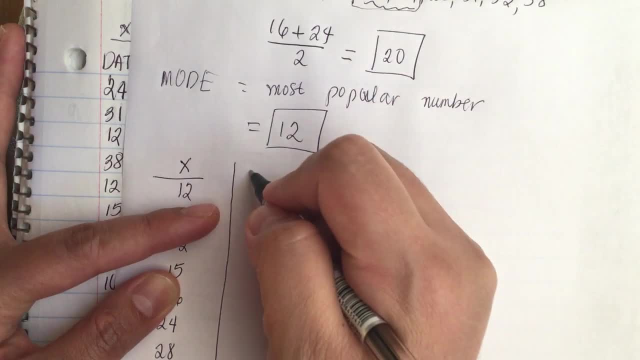 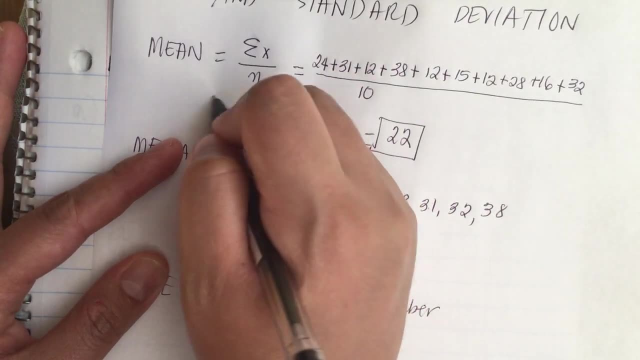 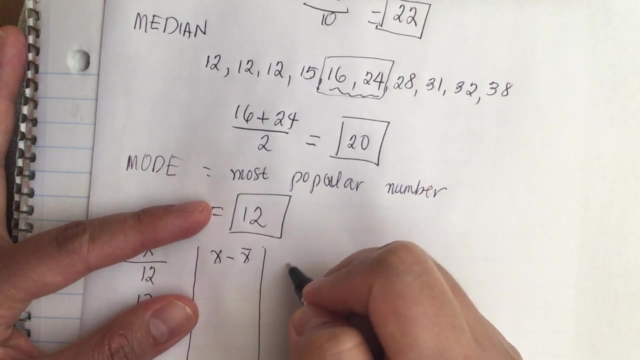 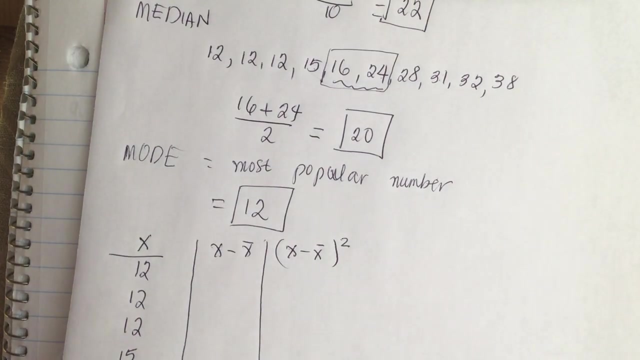 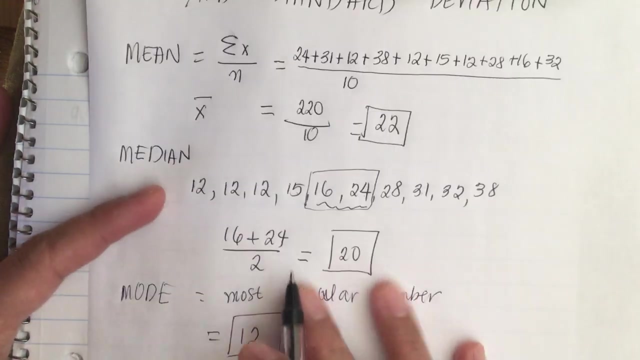 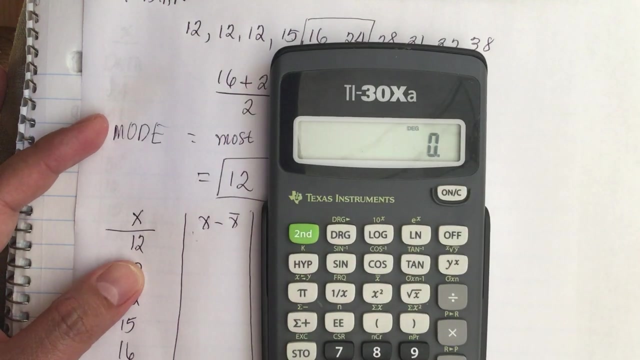 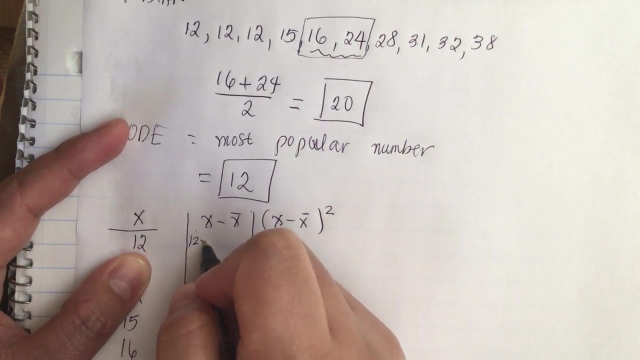 another. we need another column. so we have x minus x bar, or x bar is also called the mean. so this is the mean, x bar means mean. and then we need x minus x bar squared, so now we have 12. so we know that the mean is equal to 22.. so we have 12.. so this is equal to 12.. so x is equal to 12 minus x bar, x bar. 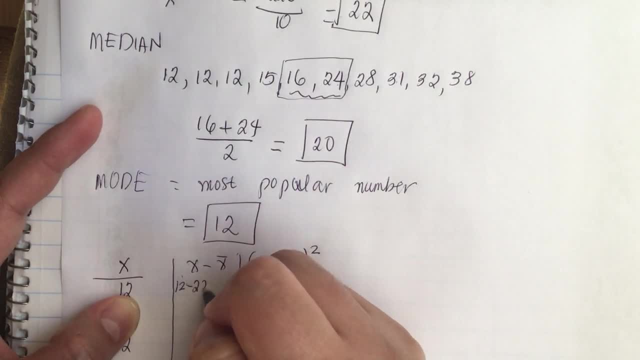 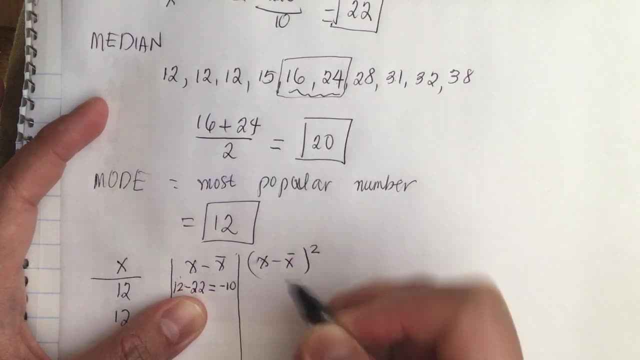 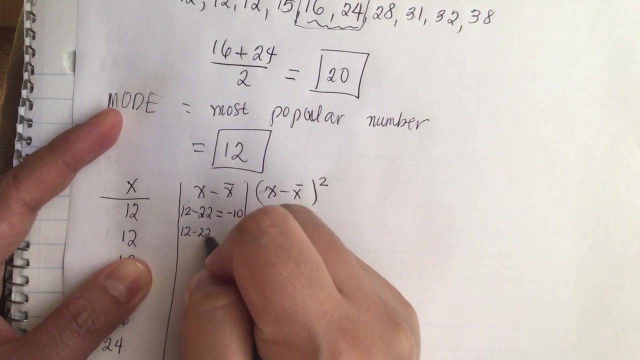 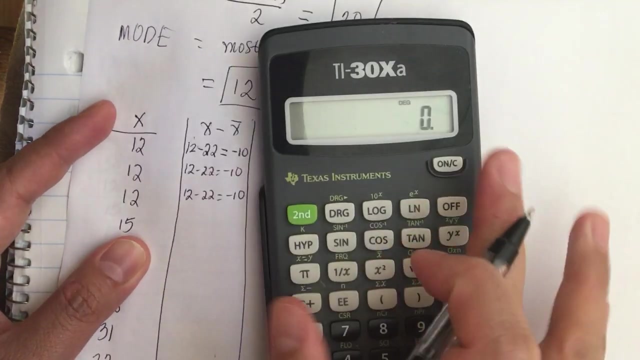 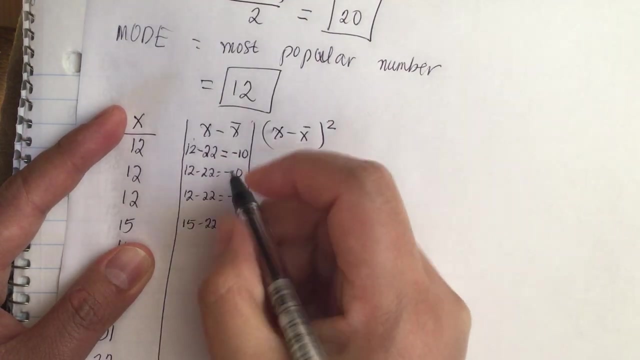 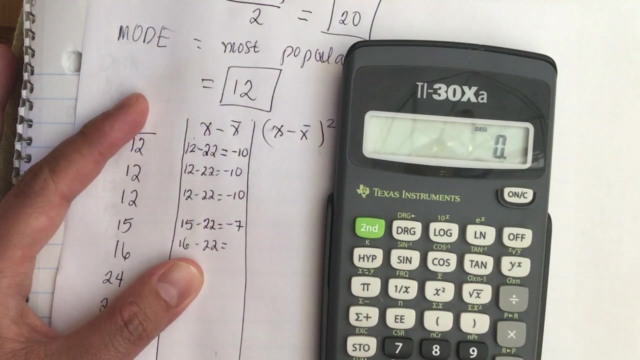 is 22.. oh okay, so this is equal to minus 10.. so this is minus 10.. these are the same: 12 minus 22 is equal to minus 10.. so 12 minus 22 equals minus 10.. now, 15 minus 22 is minus 7.. so 15 minus 22 equals minus 7 and 16 minus 22. so 16 minus 22 equals minus. 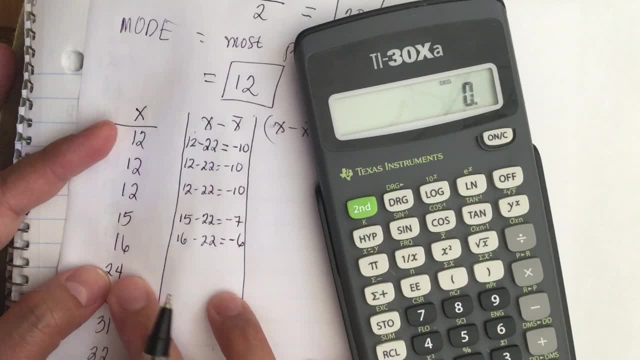 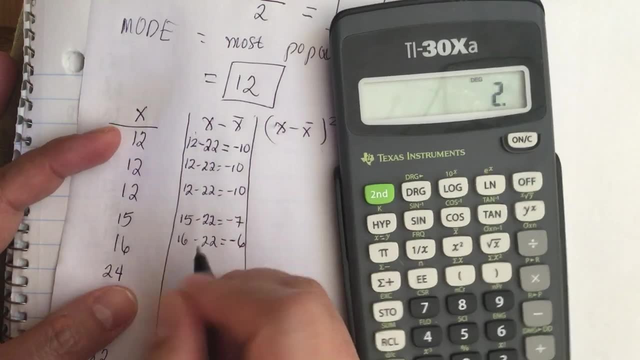 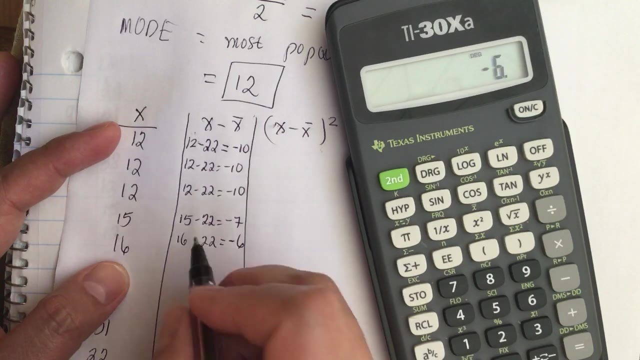 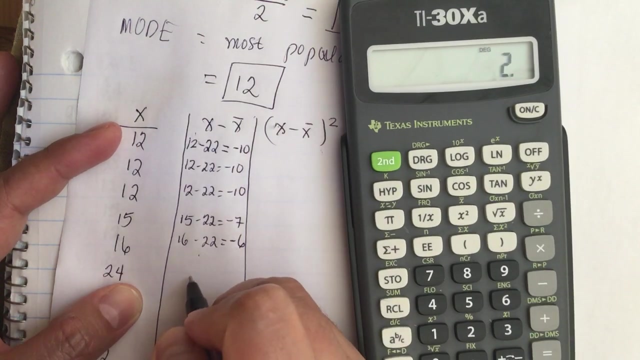 6. now in here. so we have 24 minus 22, so it's equal to 2.. 16 minus 22 is minus 6.. so now then we have: 24 minus 22 is 2.. so i just write down 2 here this: 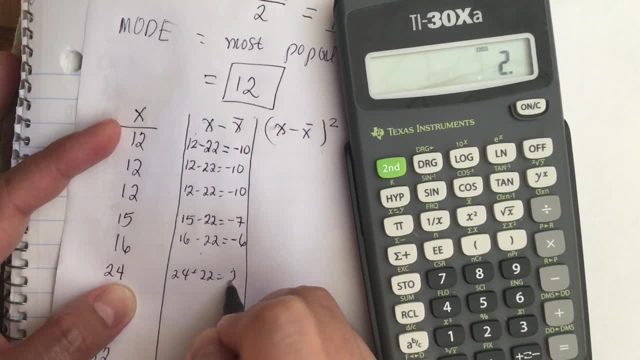 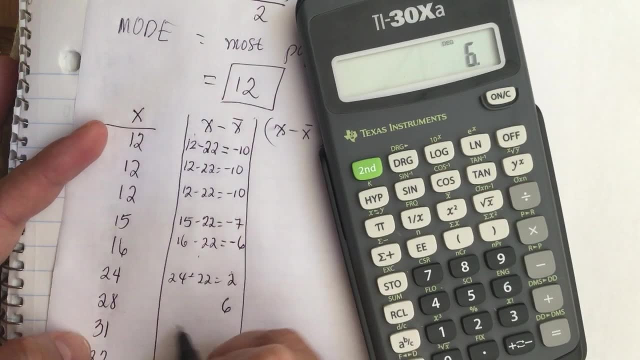 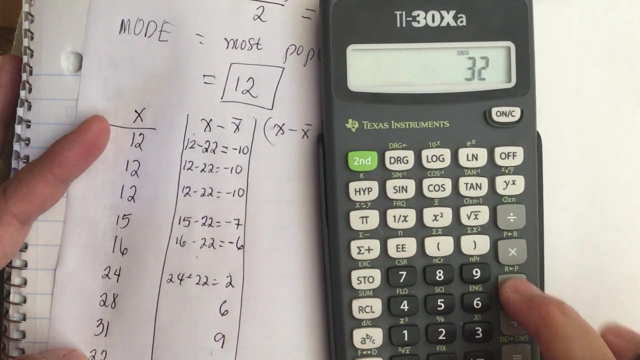 is um 24 minus 22 is equal to 2.. so i just write down 2 here. this is um: 24 minus 22 is equal to 2.. so 28 minus 22 is 6.. so this is 6.. then 31 minus 22 is 9, and then 32 minus 22 is 10. 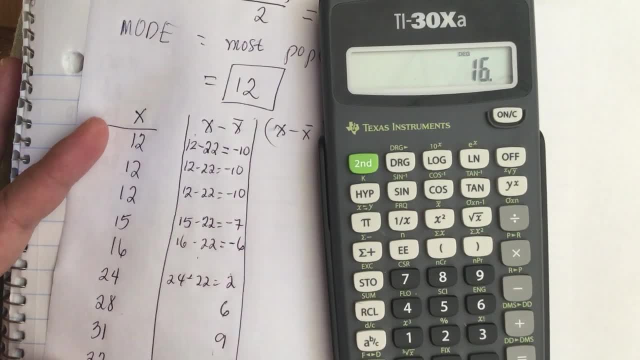 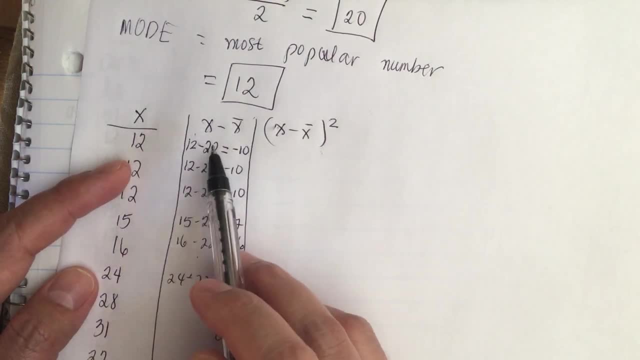 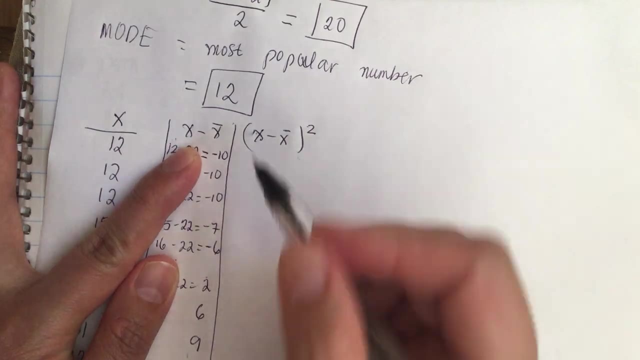 and then 38 minus 22 is 16.. so this is how you do: x minus x bar, so 12 minus the mean. so now we square x minus x bar. this means that minus 10 times minus 10, so we have minus 10 times minus 10. this. 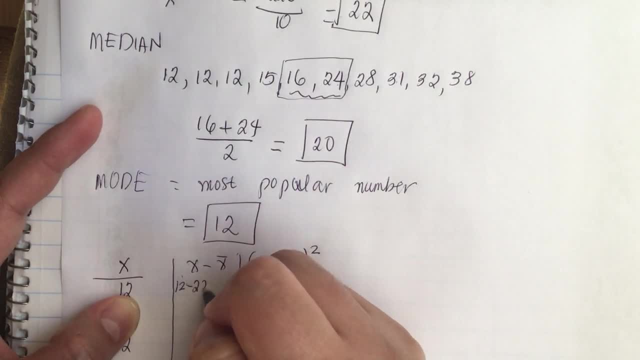 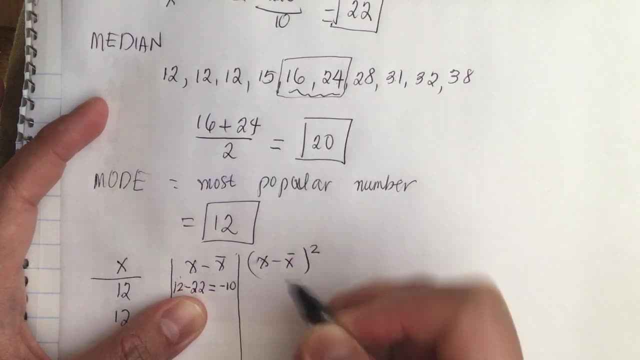 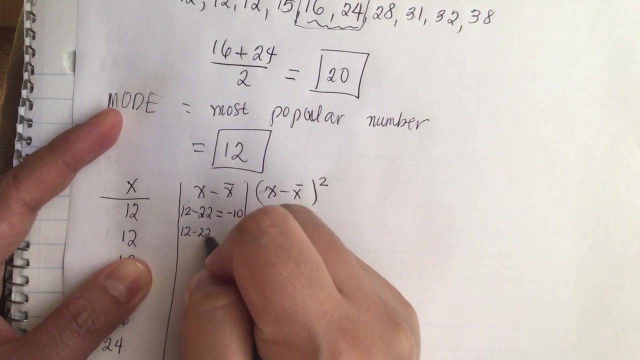 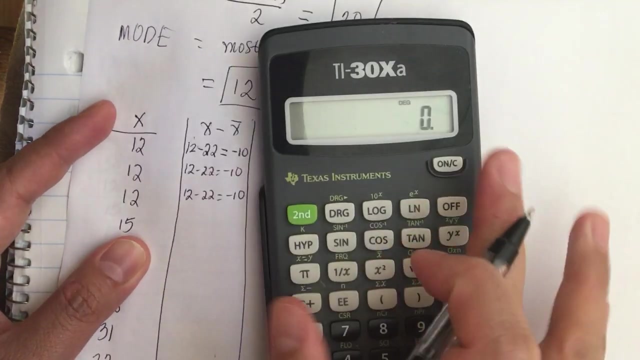 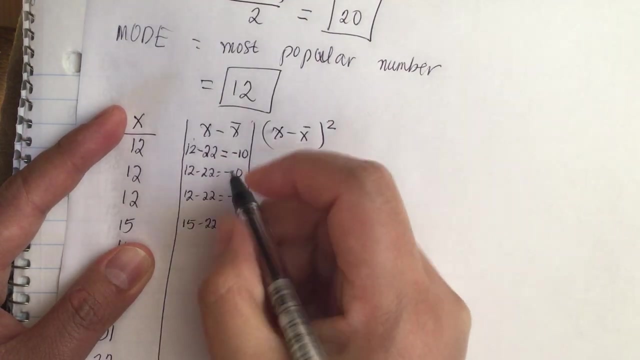 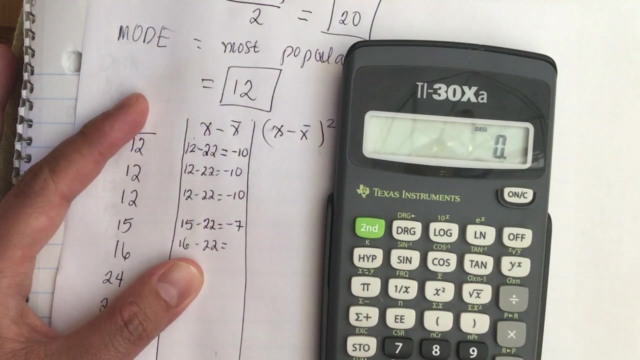 is 22.. oh okay, so this is equal to minus 10.. so this is minus 10.. these are the same: 12 minus 22 is equal to minus 10.. so 12 minus 22 equals minus 10.. now, 15 minus 22 is minus 7.. so 15 minus 22 equals minus 7 and 16 minus 22. so 16 minus 22 equals minus. 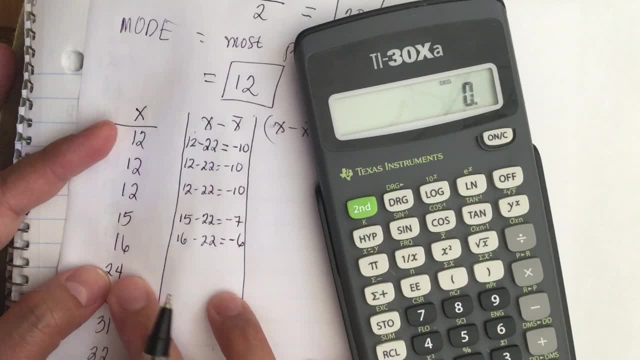 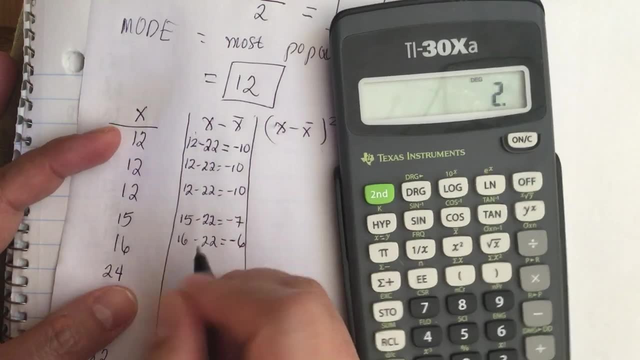 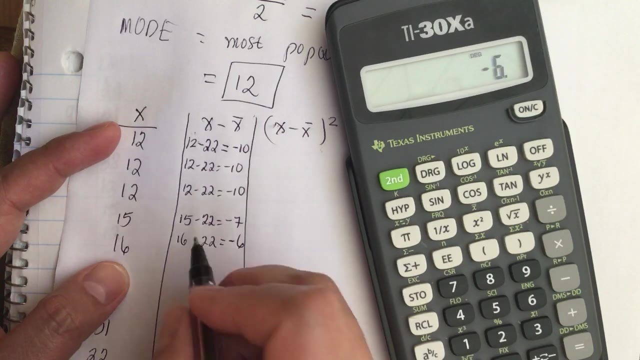 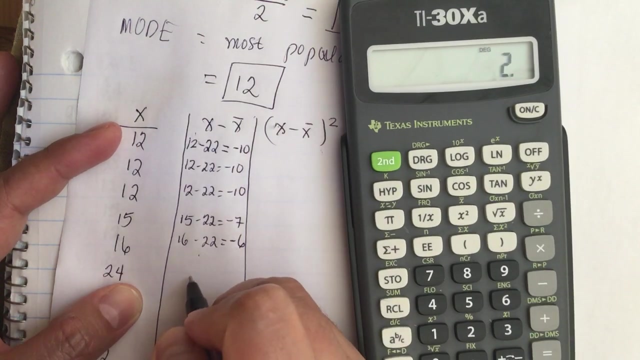 6. now in here. so we have 24 minus 22, so it's equal to 2.. 16 minus 22 is minus 6.. so now then we have: 24 minus 22 is 2.. so i just write down 2 here this: 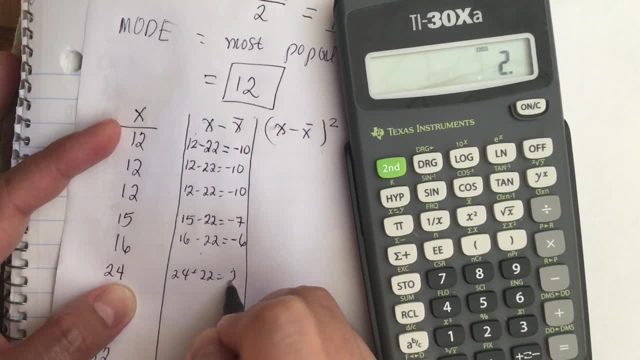 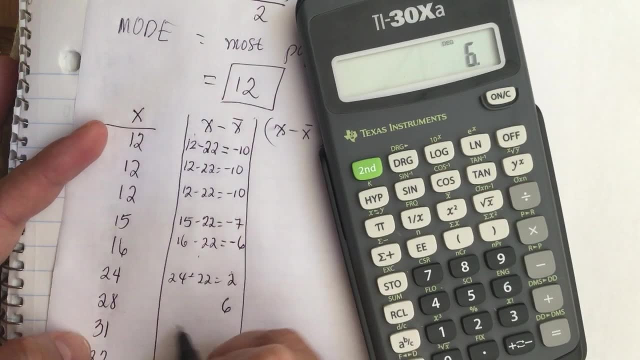 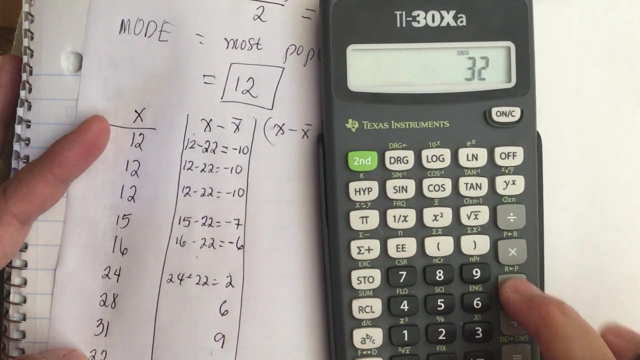 is um 24 minus 22 is equal to 2.. so i just write down 2 here. this is um: 24 minus 22 is equal to 2.. so 28 minus 22 is 6.. so this is 6.. then 31 minus 22 is 9, and then 32 minus 22 is 10. 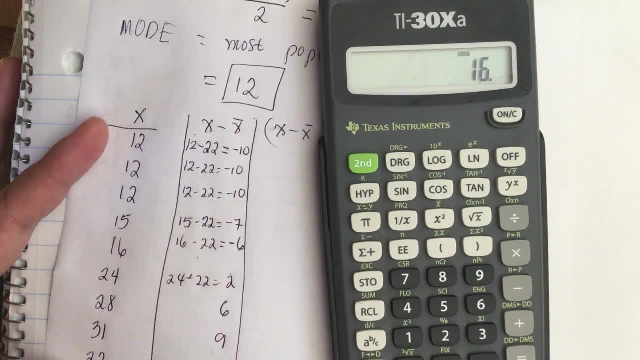 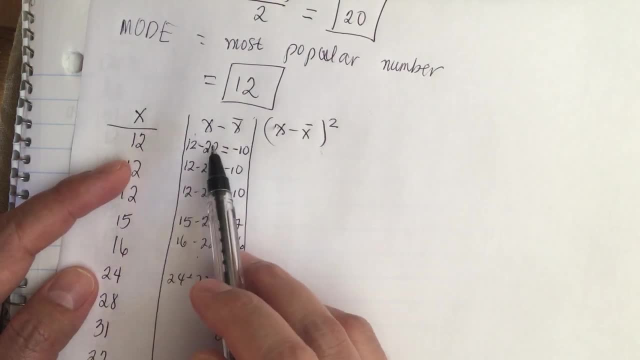 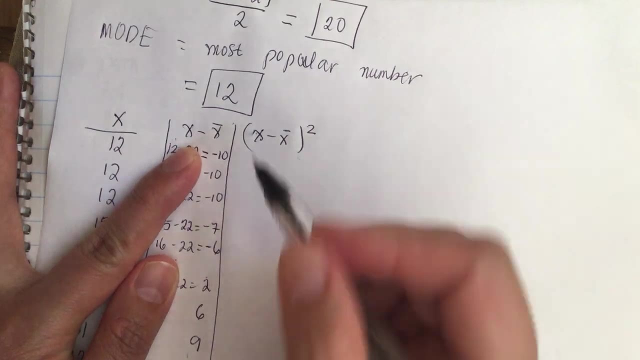 and then 38 minus 22 is 16.. so this is how you do: x minus x bar, so 12 minus the mean. so now we square x minus x bar. this means that minus 10 times times minus 10.. so we have minus 10. 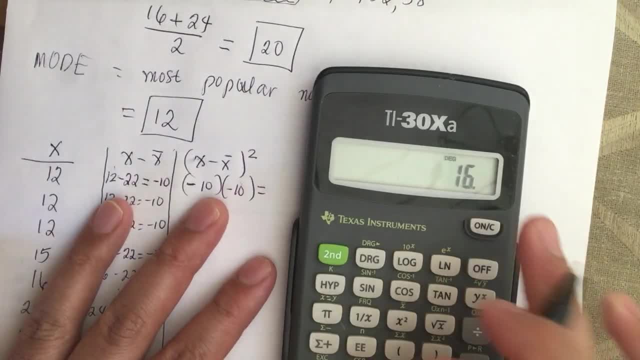 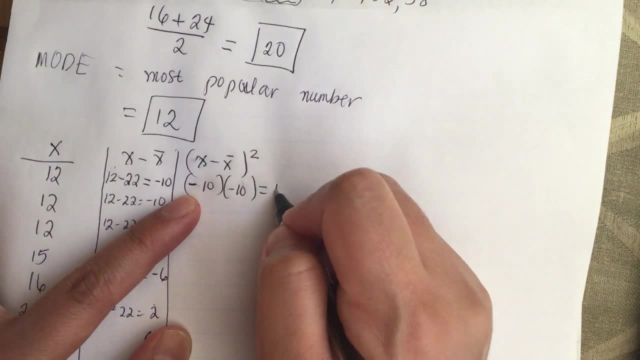 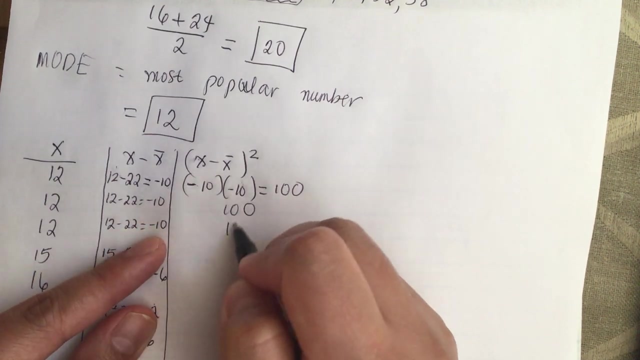 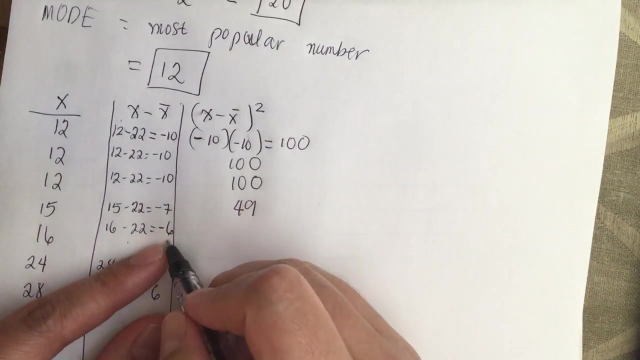 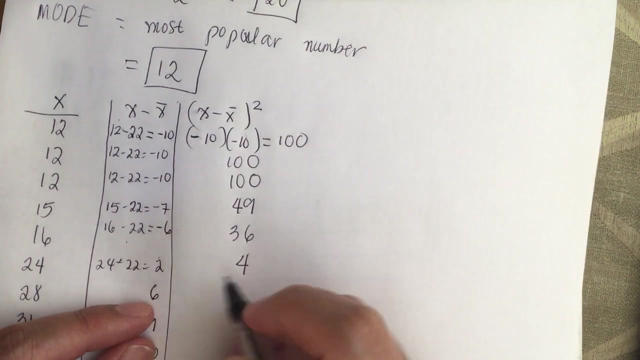 times minus 10. this is what square means. so 10 times 10 is a 100 and there are two minus signs, so it's positive. so basically you just square the number. so this is 100, so that means this is also 100 and this is 100. and 7 times 7 is 49, and 6 times 6 is 36, and then 2 times 2 is 4, and then 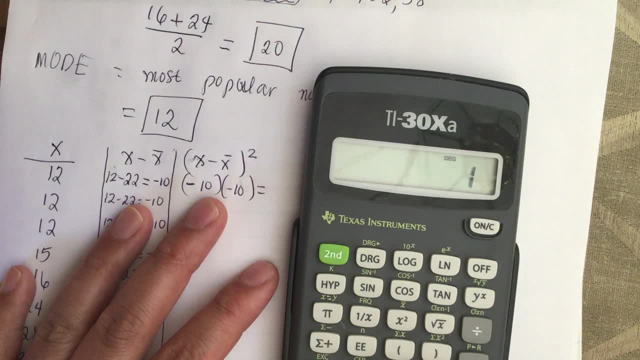 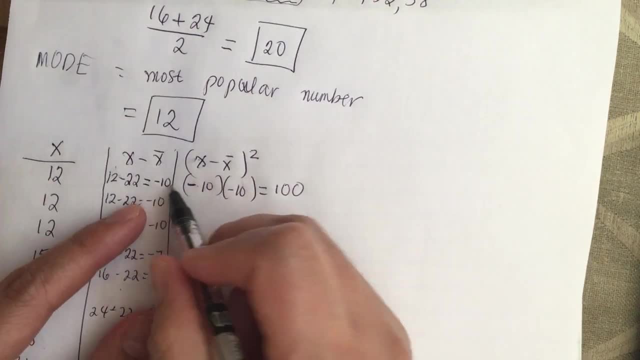 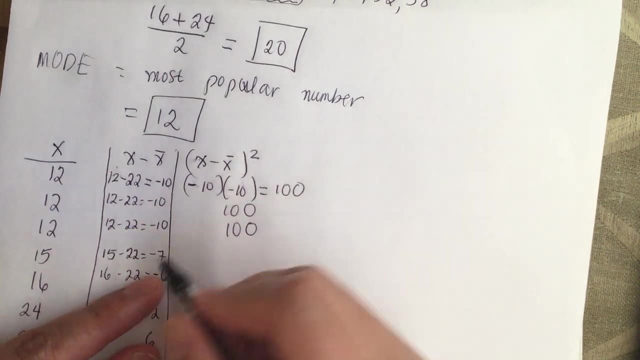 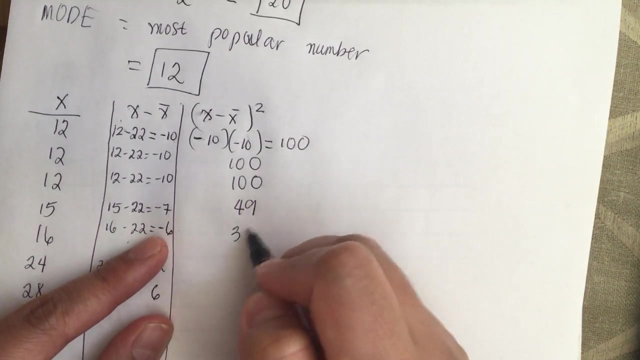 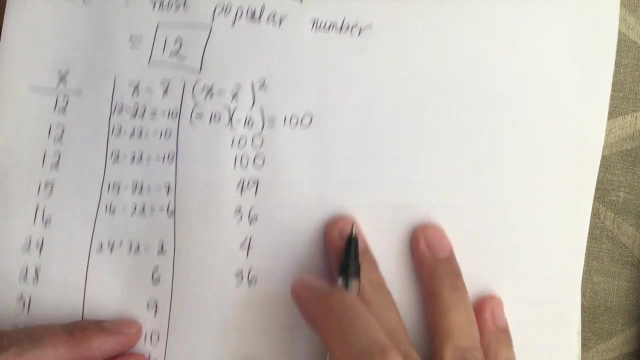 is what square means. so 10 times 10 is a 100 and there are two minus signs, so it's positive. so basically you just square the number. so this is 100, so that means this is also 100 and this is 100. and 7 times 7 is 49, and 6 times 6 is 36, and then 2 times 2 is 4, and then 6 times 6 is 36. 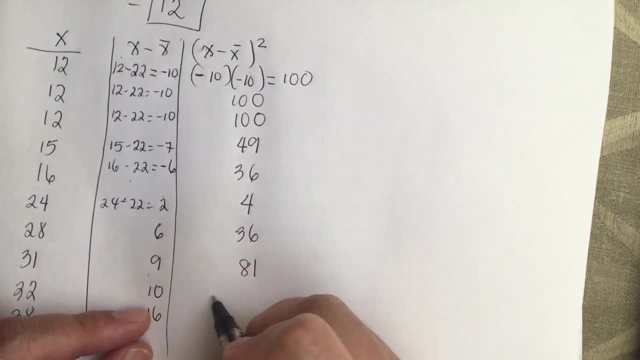 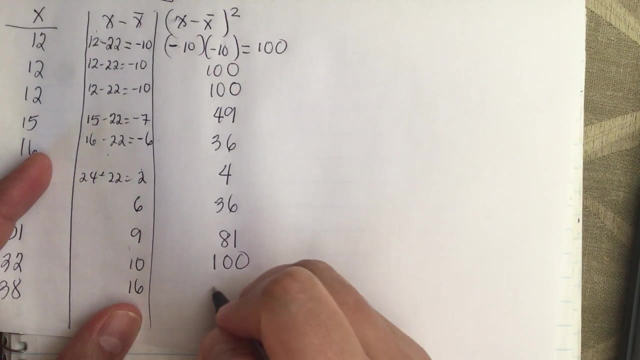 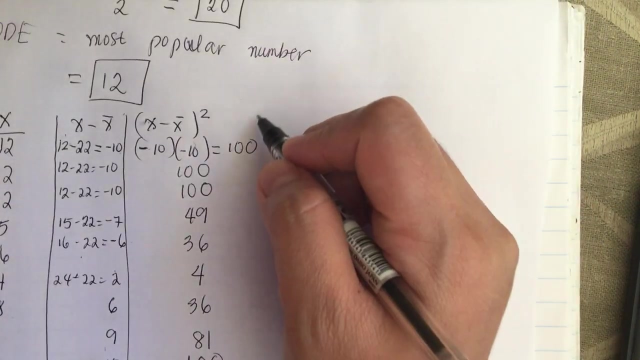 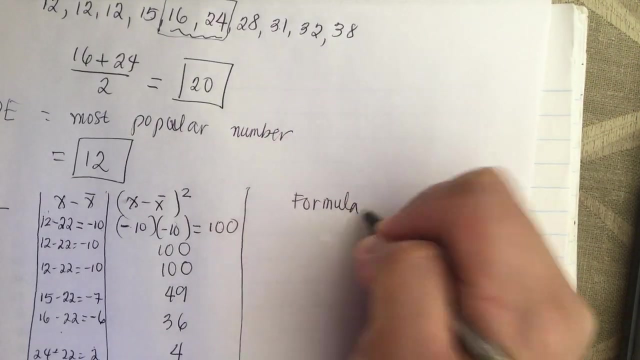 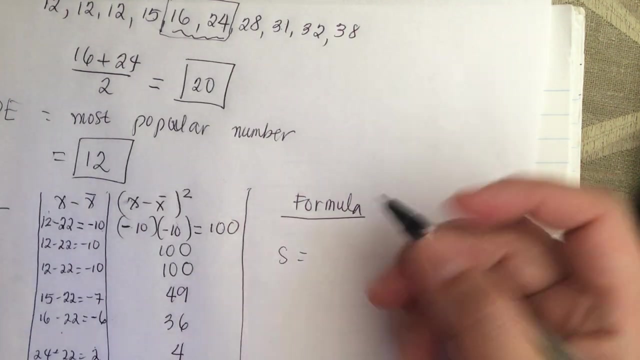 9 times 9 is 81, and then 10 times 10 is 100, and 16 times 16 is equal to 256. so, and then we need the sum. so the formula for standard deviation is equal to s is equal to s for standard deviation for sample, the sum, so the 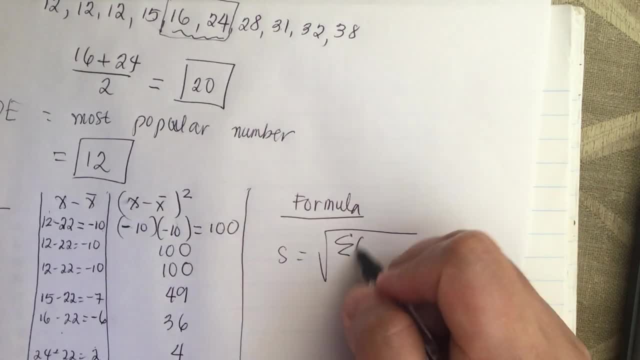 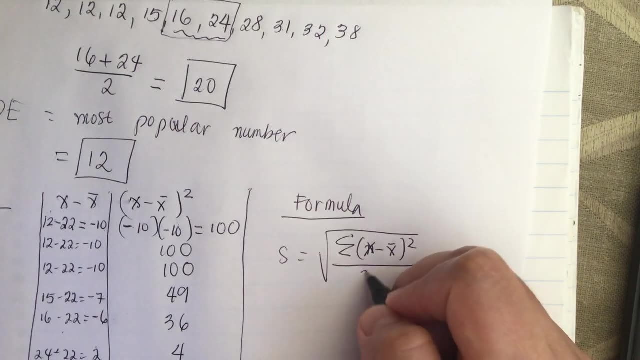 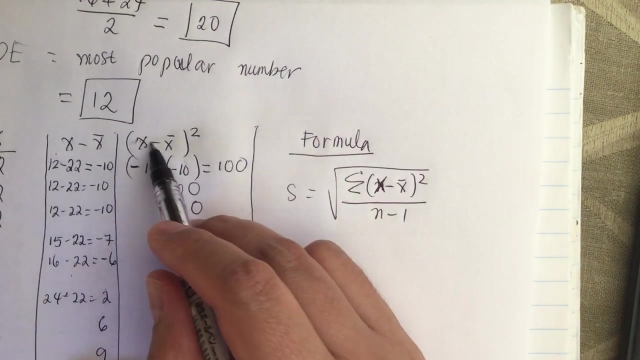 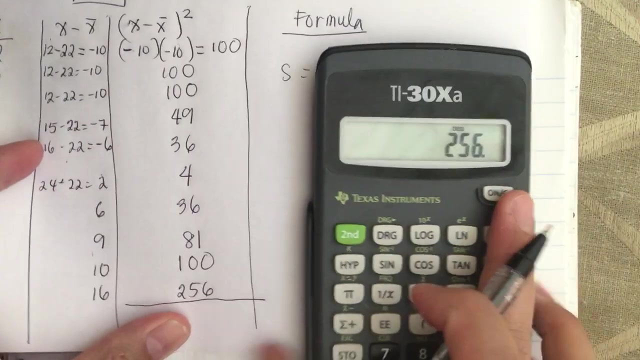 square root of the sum of x. i use x, so x minus x bar squared all over n minus 1. so we need to sum x minus x bar squared. so this is the column x minus x bar squared. so we need to sum this. so we add this, so we have 100. 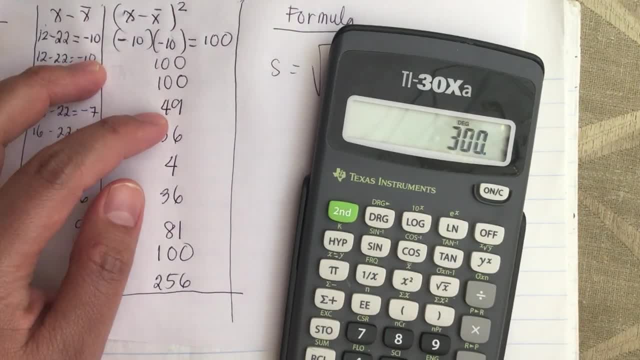 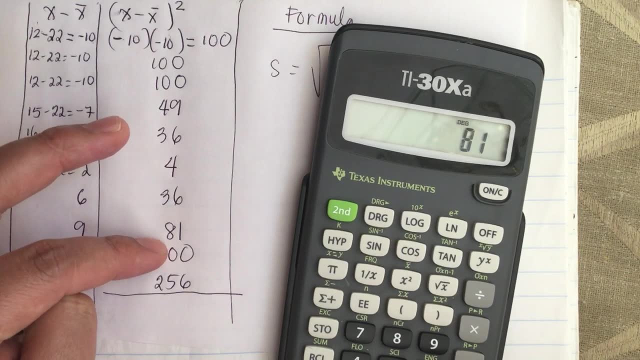 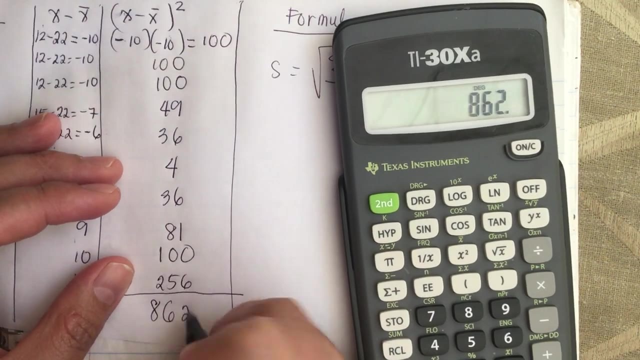 plus 100 plus 100 is 300 plus 49 plus 36, so we have 100 plus 100 plus 100 is 300 plus 49 plus 36 plus 4 plus 36 plus 81 plus 100 plus 256 is equal to 862. so now we just plug in into the. 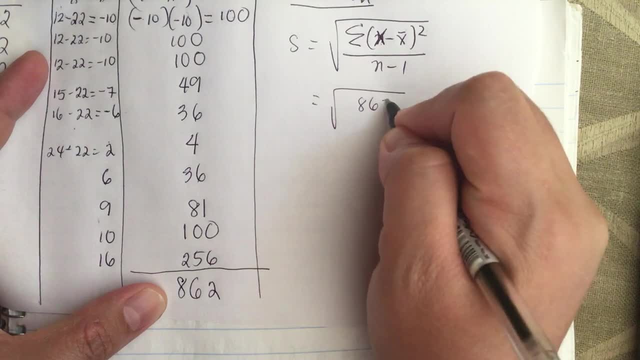 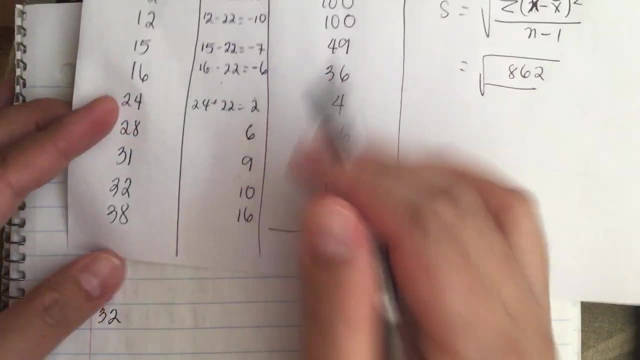 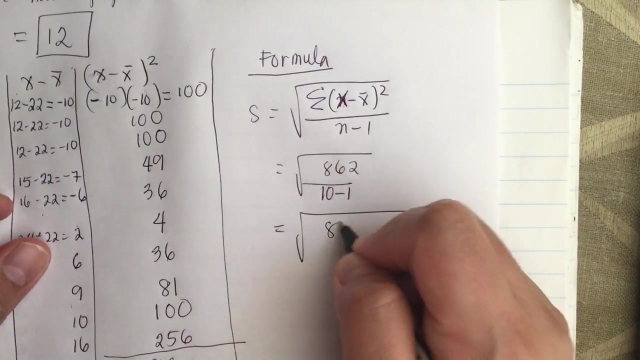 formula. so the square root of 862 all over n is equal to 10. we know that. so there are 10 data points. so 10 minus 1. so you got 10 minus 1. so this is equal to 862 over 9. so this is equal to. 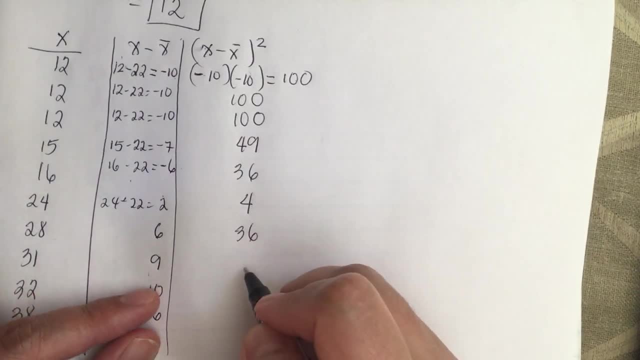 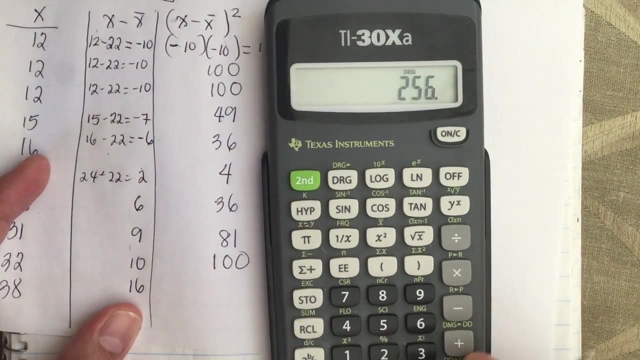 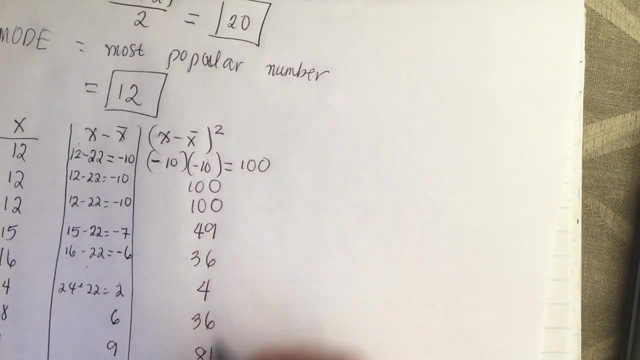 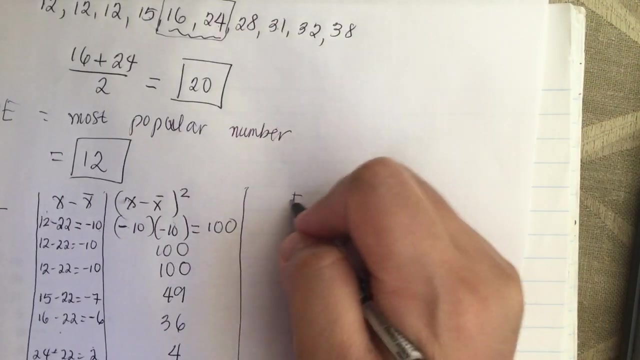 6 times 6 is 36, 9 times 9 is 81, and then 10 times 10 is 100, and 16 times 16 is equal to 256. so, and then we need the sum. so the formula for standard deviation is equal. 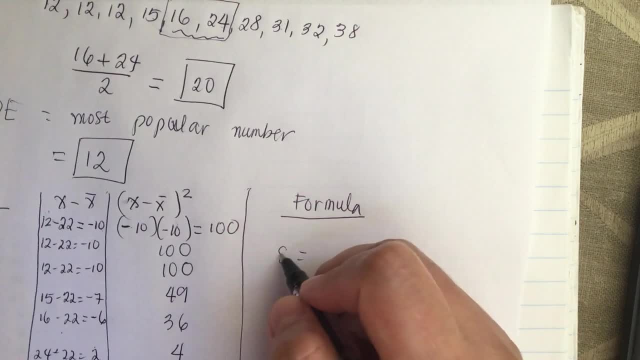 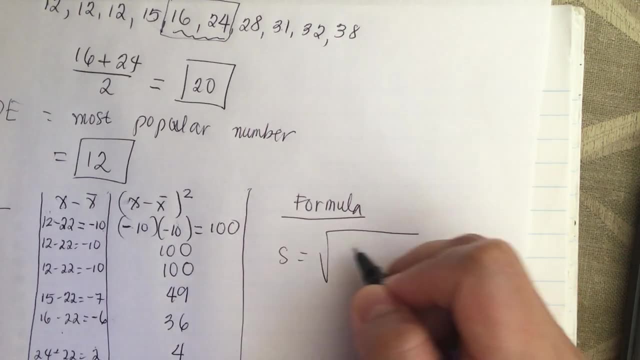 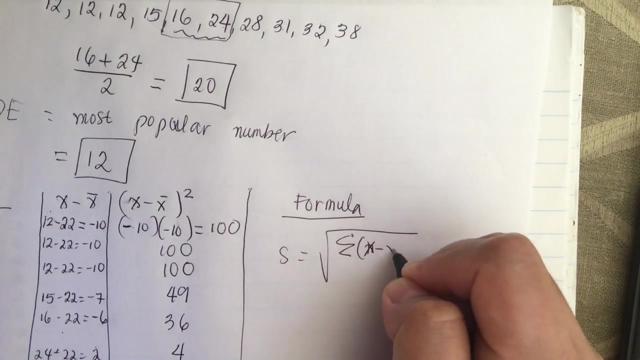 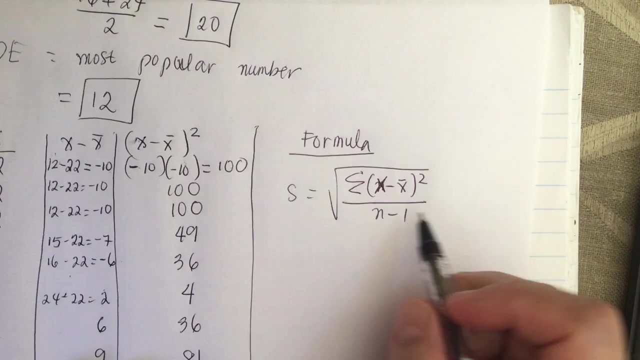 to s is equal to s for standard deviation. for sample, the sum, so the square root of the sum of X. I use X. so X minus X bar squared all over n minus 1. so we need to sum X minus X bar squared. so this is the column: X minus X bar squared. so we need to sum. 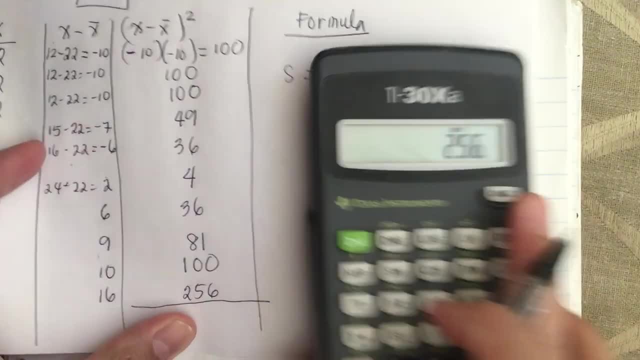 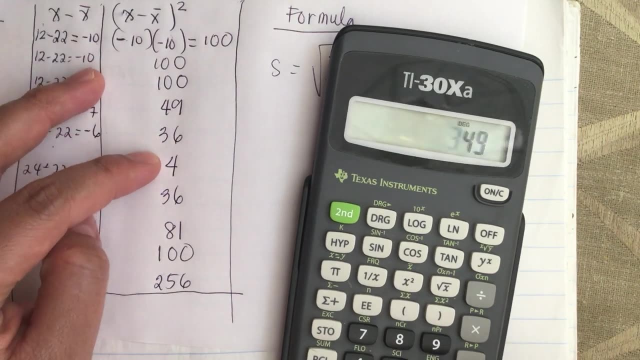 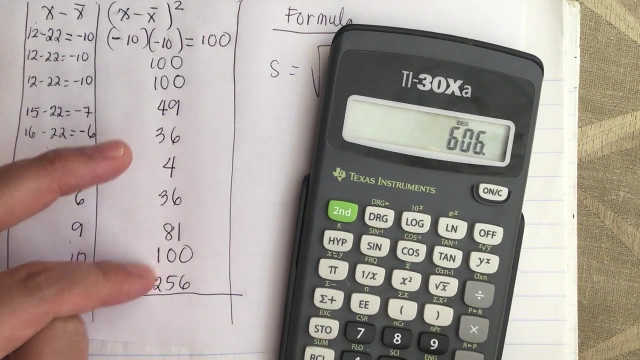 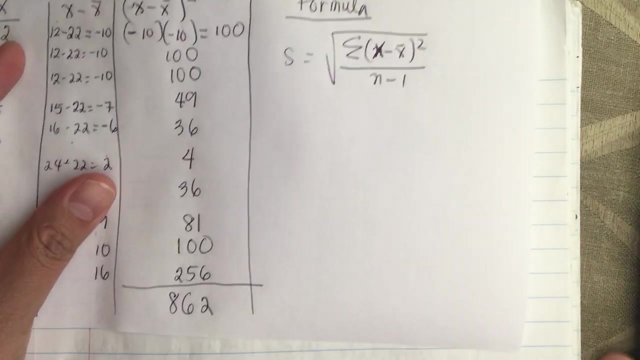 this. so we add this, so we have 100 plus 100 plus 100 is 300 plus 49 plus 36 plus 4 plus 37 plus 81 plus 100 plus 256 is equal to 862. so now we just plug in into the um formula. so the square. 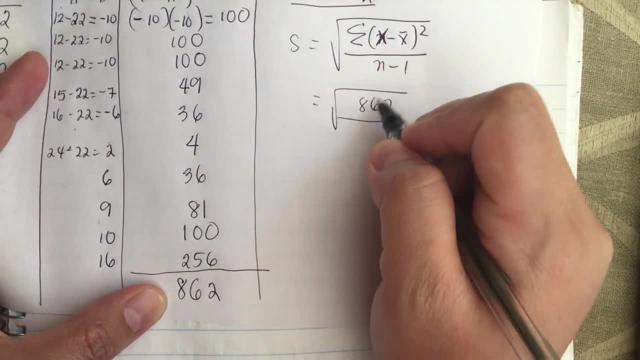 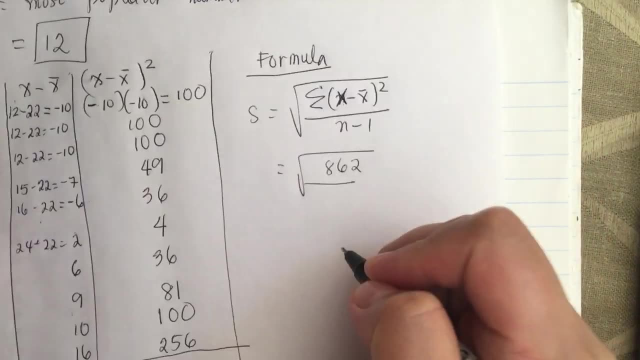 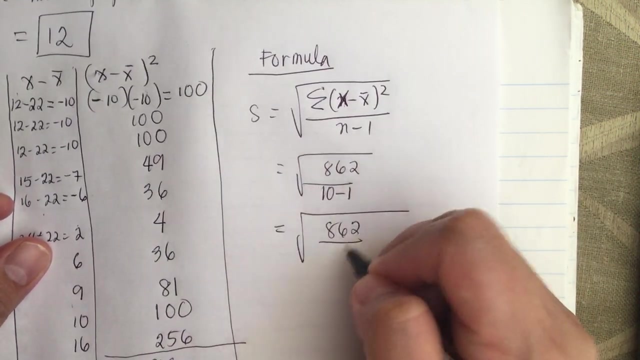 root of 862 all over n is equal to 10. we know that. so there are 10 data points. so 10 minus 1. so you got 10 minus 1. so this is equal to 862 over 9. so this is equal to. 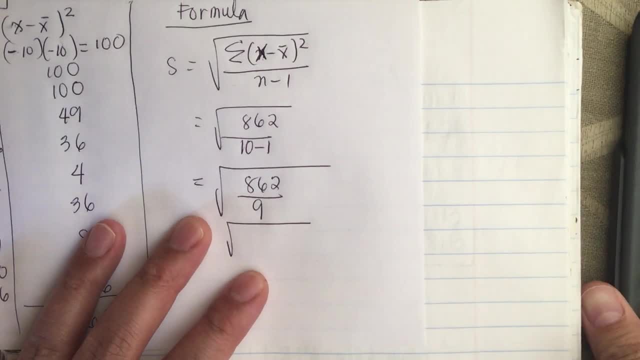 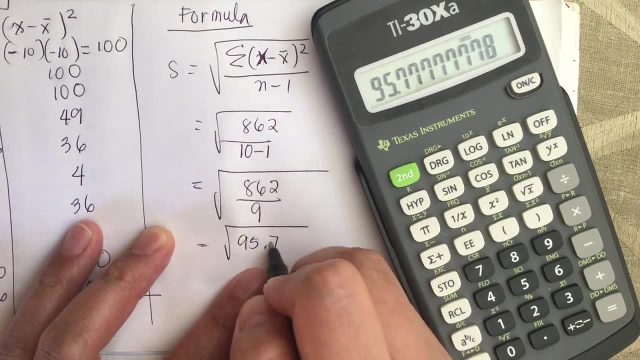 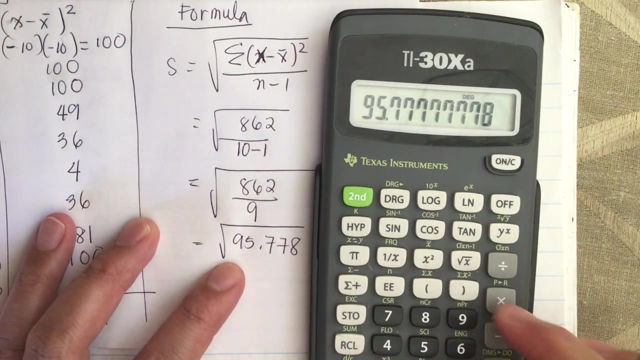 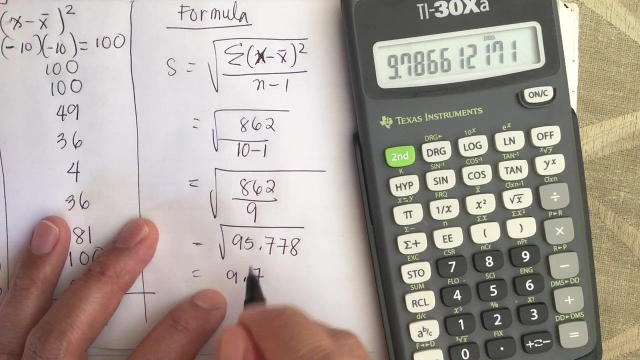 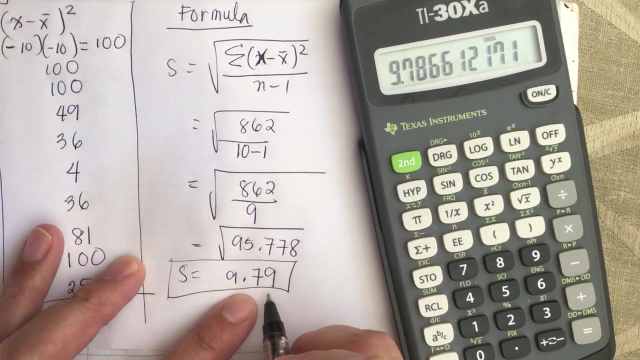 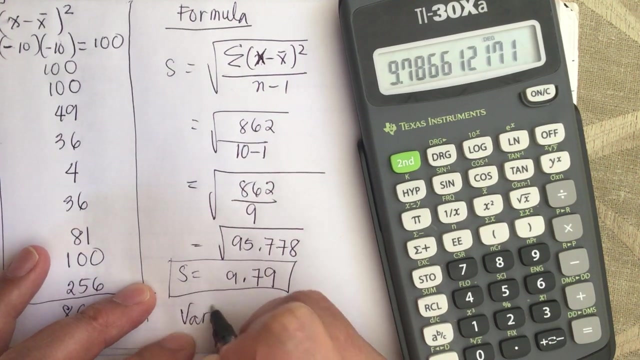 um 95.77, say 8. so now we take the square root of this and it's equal to 9.79. so the standard um deviation is equal to 9.79. now the variance is the square of the standard deviation. so variance is equal to the square of standard deviation. so